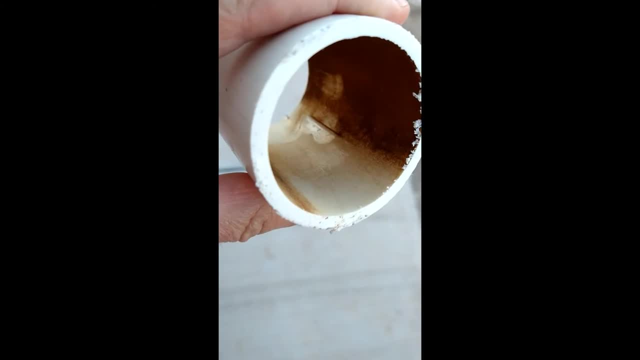 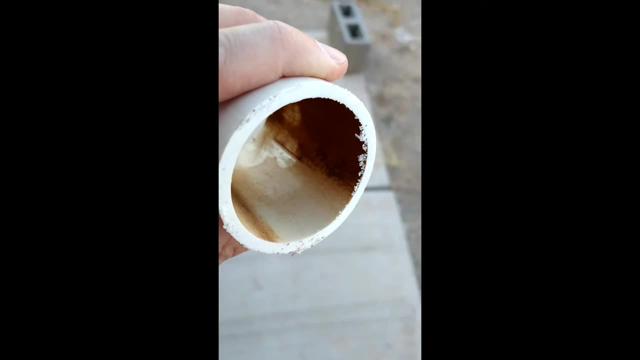 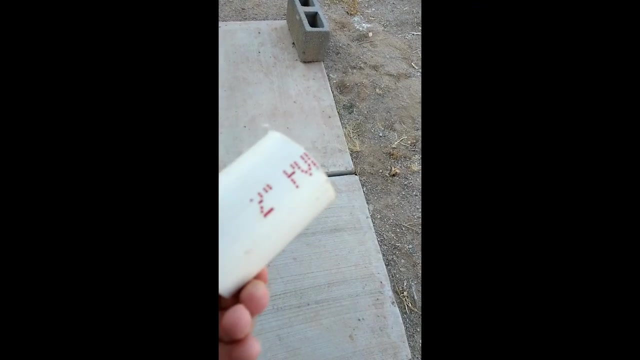 I'm talking about failure analysis and this is an example of failure analysis done to a processing problem And this has really been the bane of my existence. So you see that little groove there in this PVC pipe that I had, in my two-inch PVC pipe that I had in my front yard there. 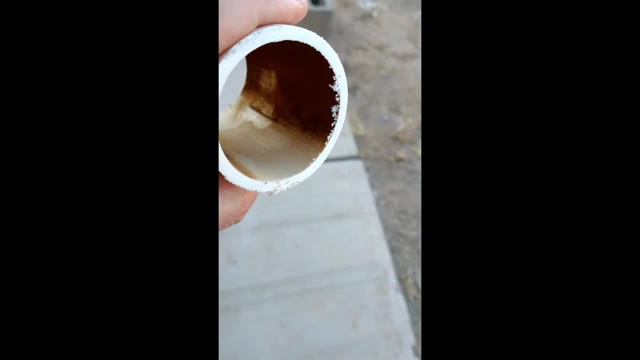 and it's led to several leaks, because this is probably a problem with the processing equipment, And so this little defect shows up every so often on the length of the pipe and it ends up being a weak point, And you just think about hoop stress, And so I start getting longitudinal cracks. 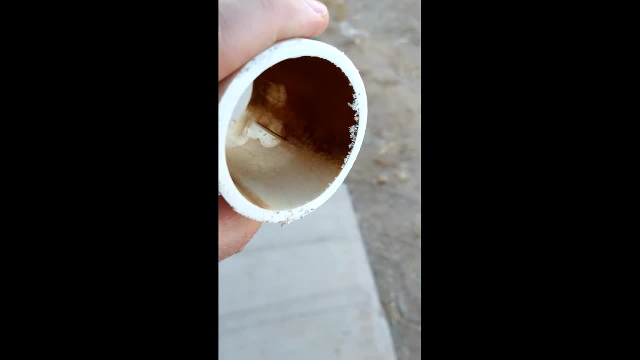 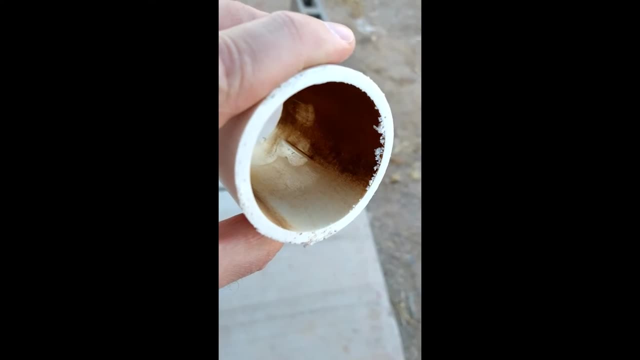 and it leads to leaks And I'll kind of show you a picture of the carnage that this leads to. but stuff like this lately has been the bane of my life. It falls definitely in the category of polymer failure analysis, but this is a failure caused by. 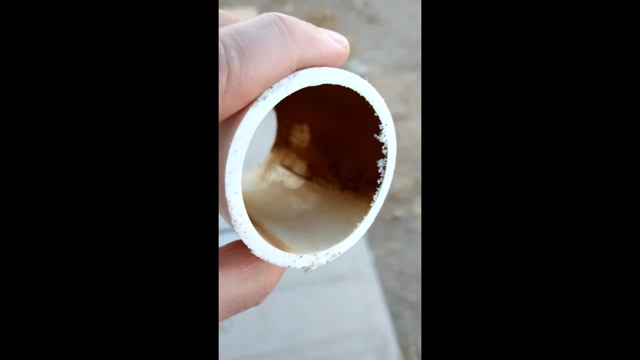 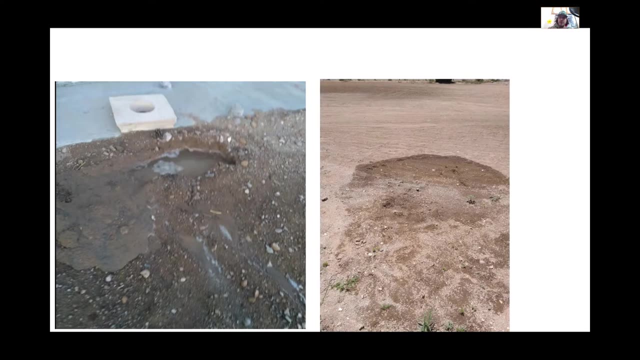 the actual processing and extruding the pipe. All right, so we saw the video and the picture here. Let me get my fancy laser pointer. This is a little blurry, I think, because I was like shaking with anger because this was the 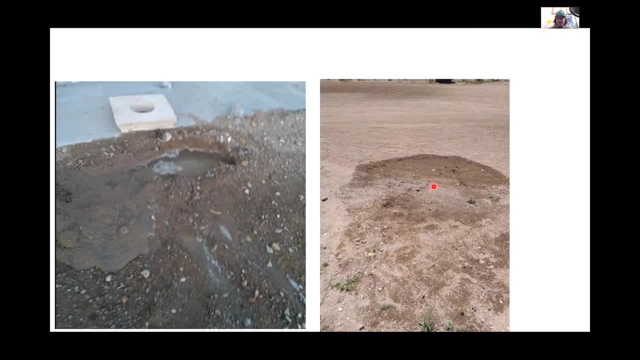 first one, actually, and you kind of see the way it's shaking. This is the water gurgling to the top. I may have mentioned it before. I live in kind of a rural area. I have a rural property, And so there's a pipe that a previous owner of the 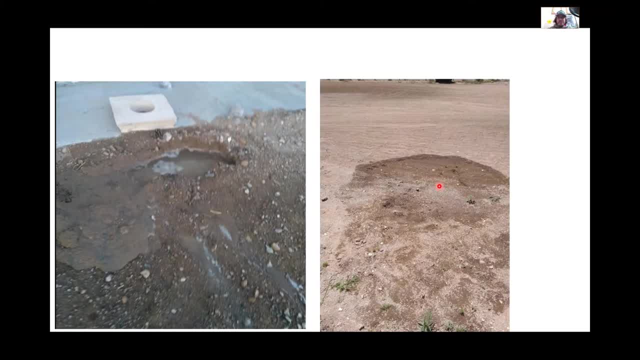 property I reside in put in kind of an auxiliary line, I think, to have more hose spigots, which was kind of interesting. I guess they couldn't buy a longer hose at Home Depot or whatever, And they actually used a pretty poor quality pipe and you saw the defect And so 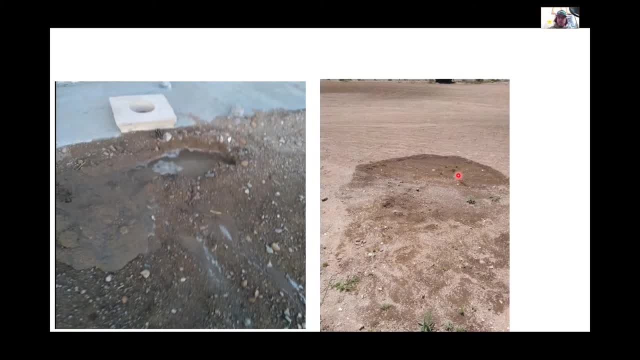 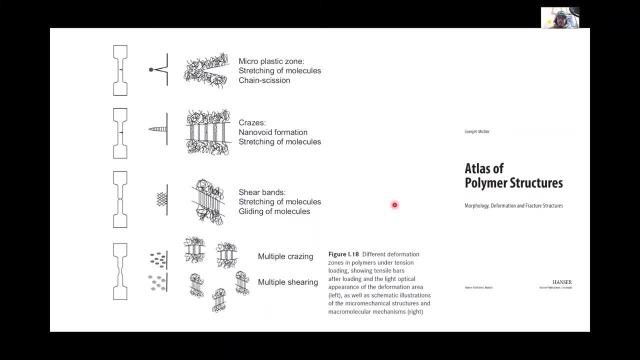 it's not the result of some polymer failure And we water gurgled here. This one was worse, But it's all the same pipe at different points and it's that recurring defect from extruding the pipe, actually extruding that PVC pipe. I got this figure from this book, Atlas of Polymer Structures. 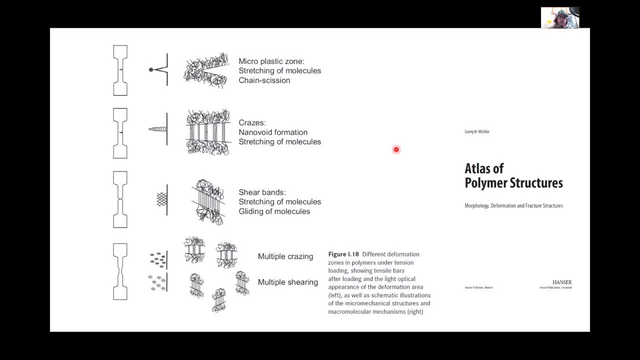 and this kind of talks about the anatomy of a failure, And so this is a tensile specimen. It's called the microplastic zone And I'm going to show this figure and I'm going to show another figure And I kind of think both of these on their own are incomplete. So this figure and the figure, 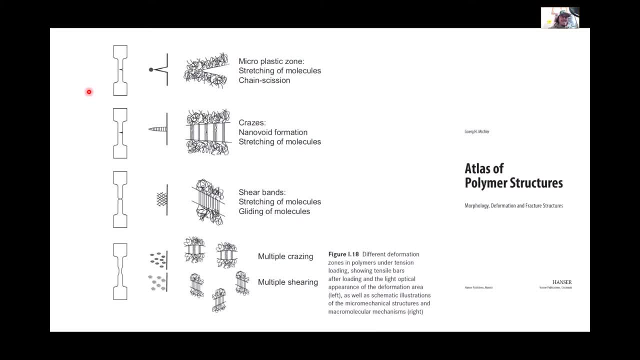 I'm going to show next. if you put the figures together, I think it kind of gives a better example of what's happening when polymers fail, basically. And so this is a dog bone tensile specimen, a little schematic. We start getting this kind of. 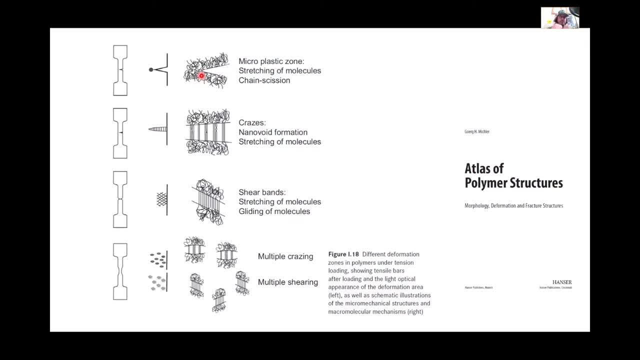 stretching of the molecule, stretching of the polymer chains. actually, Then you get chain scission And many things can cause chain scission. Moisture can actually cause chain scission. So it's important to keep at least raw polymers dry, because that can lead to a definite problem in 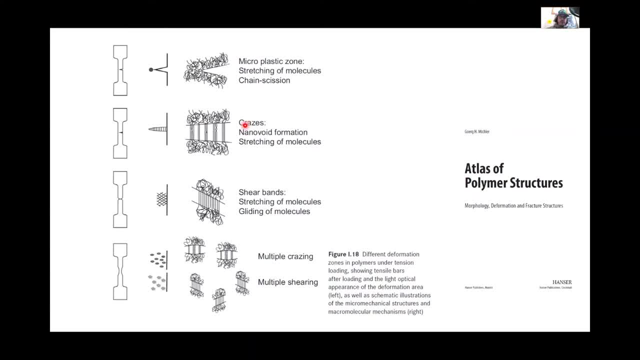 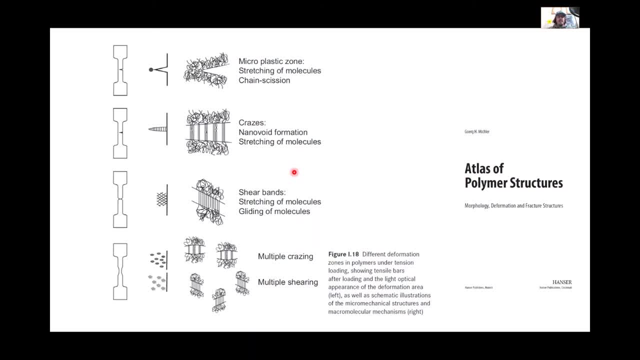 these craze cracks forming and crazing is really kind of important. It's important to grasp. anytime you bend a polymer and you see white, that's called strain whitening And that's due to a bunch of craze cracks And we'll see kind of an example here later on. But we start cutting. 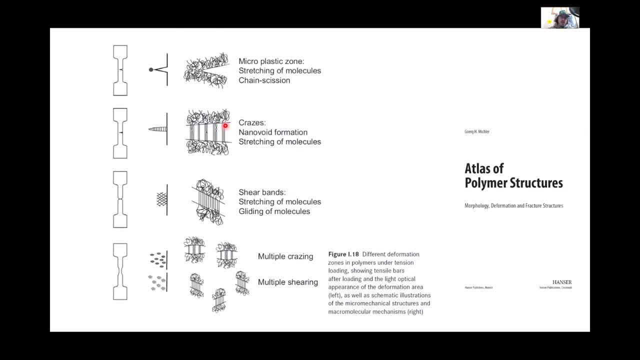 the formation of these crazes. This here I'm going to kind of kill my own reveal- When you start seeing these kind of void. so this empty space is void, where you see these kind of lines here, these elongated polymer chains. it's actually elongated polymer chains. Those are 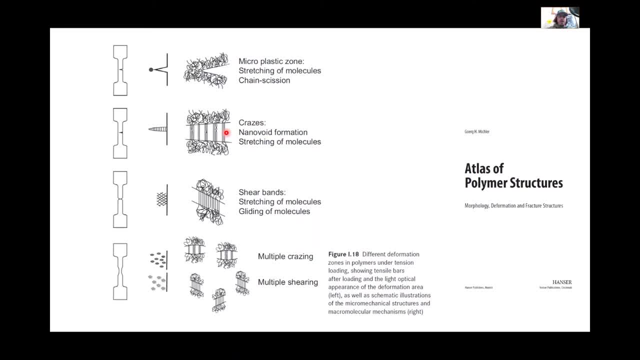 called fibrils actually, And fibrillation is kind of a big deal. We start shearing, seeing, shearing. I'm reading the slide so I kind of messed up a little bit. You start having kind of movement of the polymer change that forms what's called shear bands. 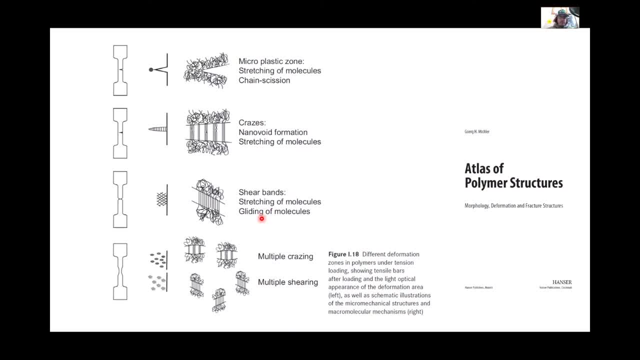 And these are actually kind of hard to see through microscopy. And then when you're starting to get necking, this is kind of nearing failure and rupture and stuff like that. I don't know why it kind of shows almost a rough ruptured area. Then it kind of shows necking here. 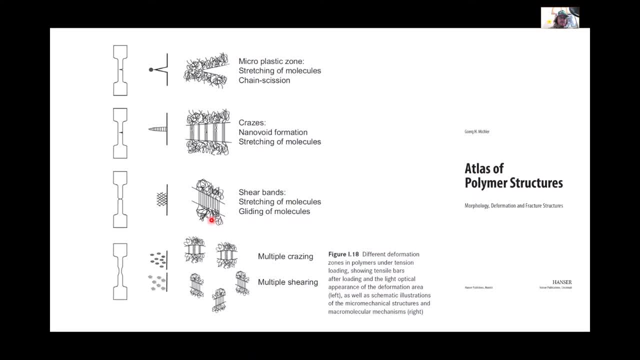 So when you have necking you have a lot of crazing And then a lot of times when you look at a tensile test you'll see kind of some white due to the craze cracks And then you get final rupture. And I don't think this is the most complete figure. No bash to this author, But 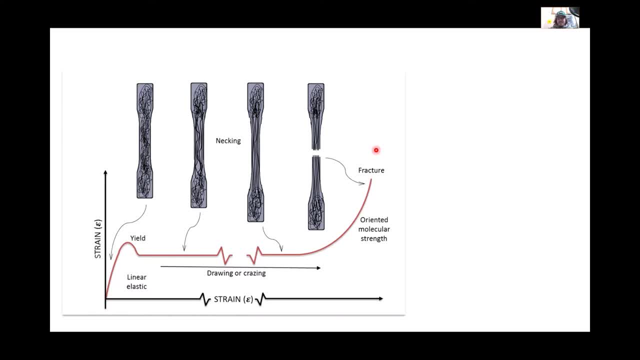 let's see this next slide. So I kind of like this figure a little better. It's missing a lot of stuff though. It's missing craze cracking and the shear band formation, But I kind of like it because it shows it in reference to a stress-strain curve, And a lot of times you get 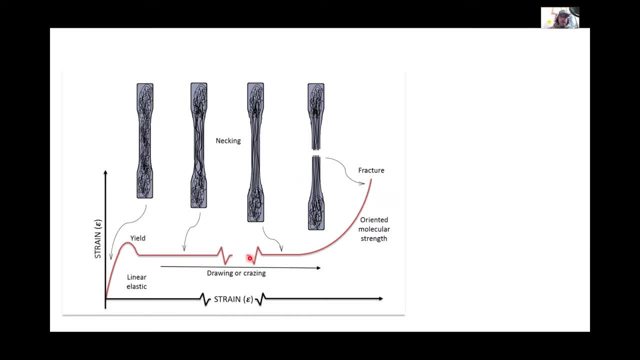 kind of this yield hump. And then you still get drawing And you still have this elongation happening. And the necking here isn't quite as dramatically depicted- I had a student draw this some time ago- But the necking is due to actually the chains elongating. And finally, 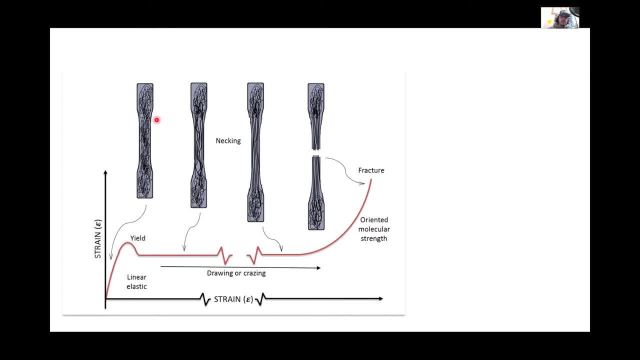 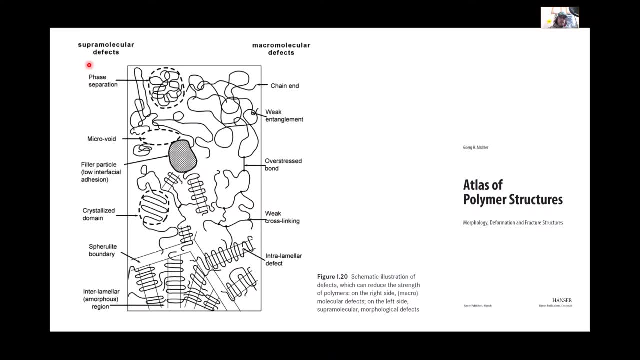 finally they break, And so we're going to see several examples of this throughout this particular lecture. This is kind of a cool figure- I really like it- And you always learn about defects, and defects related to the formation of cracks and leading to failure, particularly if you've taken failure analysis And pretty much just stress concentrators. 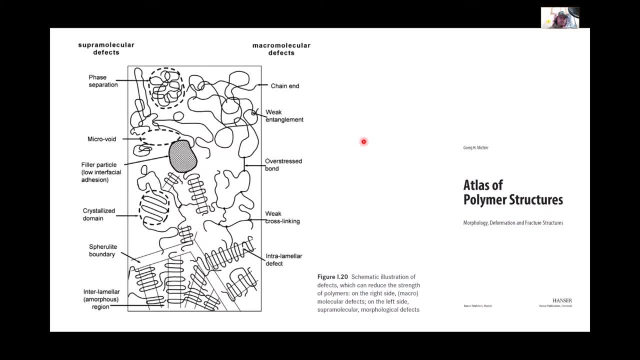 is what they end up being, And I kind of like they've kind of categorized it in two phases: Super macular and macromolecular defects And super molecular- excuse me, super molecular and macromolecular defects And kind of these different things And some of these things. 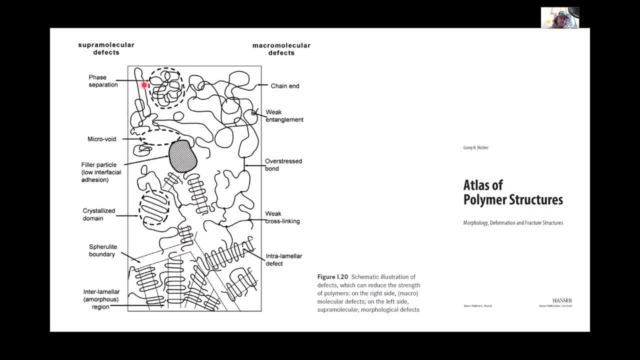 we've actually kind of talked about And phase separation. So I've shown you micrographs of polymer phases. A microvoid is pretty much just a hole. If you have a composite- and we've talked about this- And you, the interfacial adhesion of your filler material with your polymer matrix is extremely. 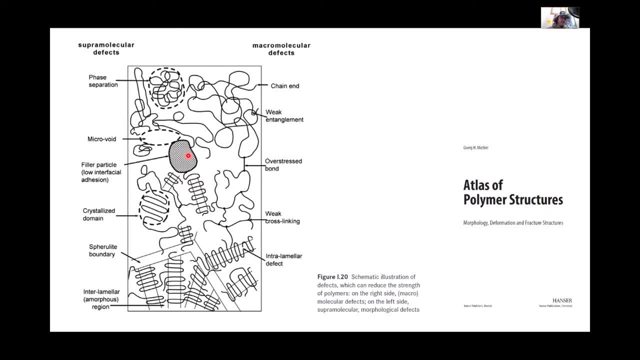 extremely important. But other stuff that you- this I would kind of call pretty obvious: The presence of a void, The presence of a filler material, Maybe even phase separation, is pretty obvious. right, That's kind of general failure things, But other stuff you don't really think. 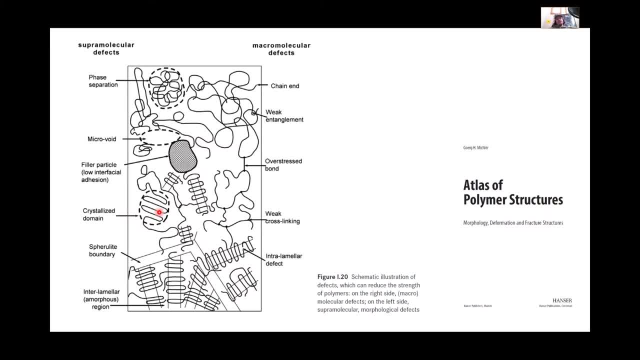 about is a crystallized domain. So we talked about crystallinity and polymer in a previous lecture And we see that the entire polymer structure is not crystalline. It's crystalline in certain spots. We have these other crystallite structures that we've talked. 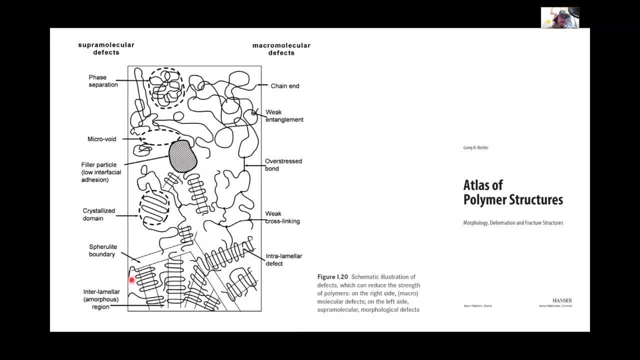 about called spherolites, And so we kind of have this represented by what doesn't really look like a spherolite. unfortunately, This little arm here kind of looks more like a spherolite. But anyway, things that aren't quite as obvious. So the interface between the crystalline and 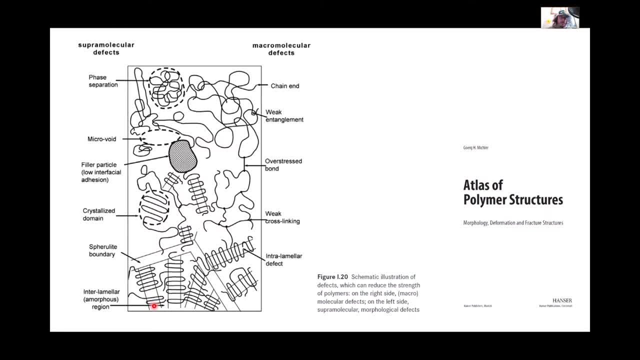 amorphous region on kind of a grander scale. Here it's kind of showing it. I said, when the polymer chains fold you have a crystalline structure altered with an amorphous kind of structure within your polymer, the holistic polymer structure, Other things that maybe. 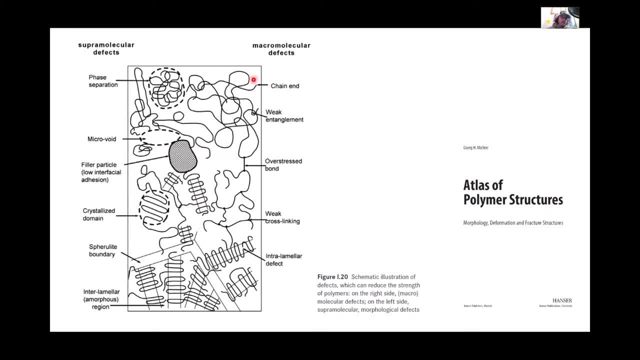 you would never think about the end of the polymer chain. So we have this kind of bowl of spaghetti type of model Where that polymer chain ends could also be a weak point Within your structure. Chain entanglement is generally good. It tends to resist. 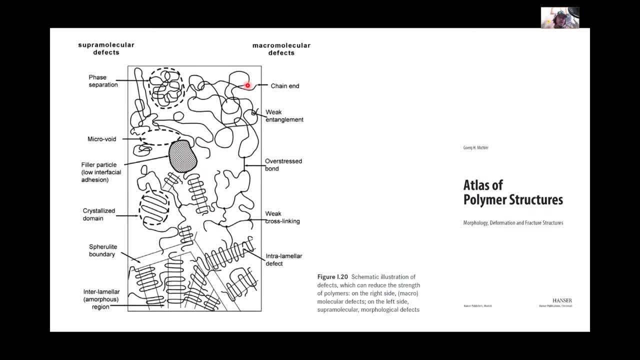 deformation if you will. But if that entanglement is weak, you have some problems there from a failure point of view, An overstressed bond. So this would be like a crosslink And we also have weak crosslinking too. So overstress, putting too much stress on your 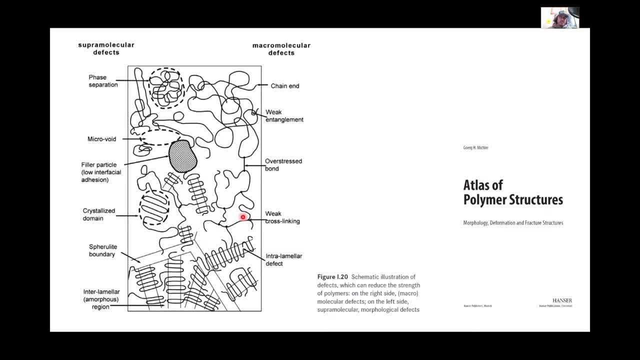 crosslink, And having your crosslinks not be strong enough could also lead to polymer failure And the strength reducing mechanism overall. And then in your crystalline domain, if you have some sort of defect in your folded polymer chain, that's another area where the strength of your material could be compromised. And so think of these things. 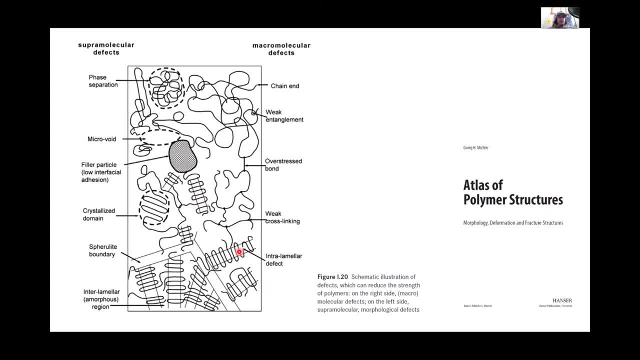 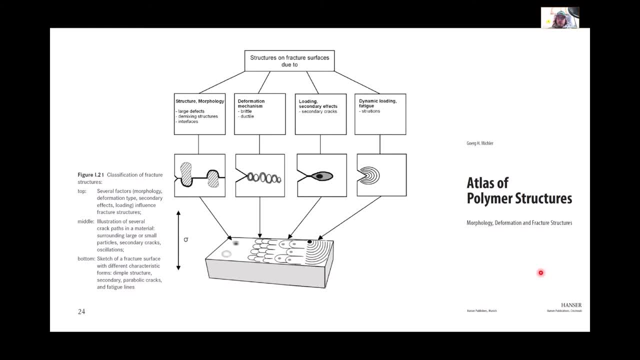 in terms of the defects within a polymer structure leading to the overall failure of your polymer structure. I kind of like this figure as well, And again I've borrowed it from this book, Michler Atlas of Polymer Structures, And it's actually kind of cool. So 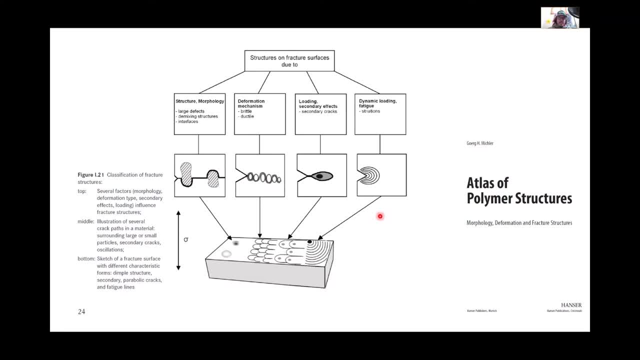 it kind of shows, kind of the schematic representation of how things look and different types of fracture morphologies, if you will. And I've written quite a few papers myself and my students on different failure analysis situations for polymers And I'll share with you. 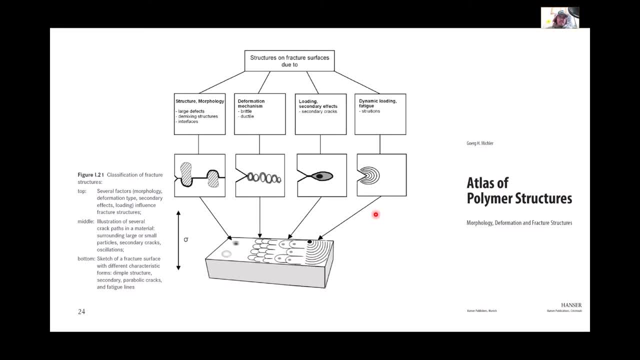 some of the figures here Again, this isn't meant to be a end, all be all course on polymer failure analysis. This is one small lecture in a greater class, But hopefully this kind of whets your appetite to kind of look further into it And maybe, if you've seen stuff like 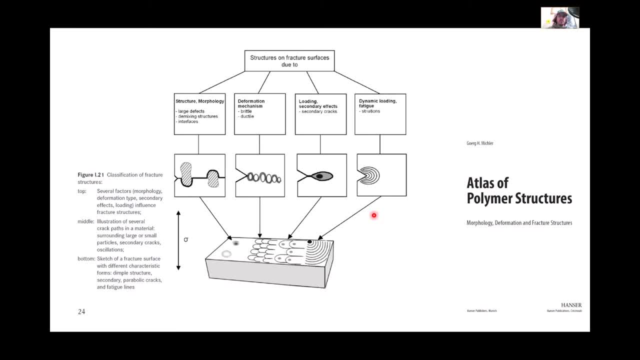 failure analysis or polymer failure analysis in the course failure analysis offered by our department. you can kind of correlate what I'm saying with that. instructor Dr Stafford um says in his course as well: uh, but it's kind of cool. so you know large defects um. 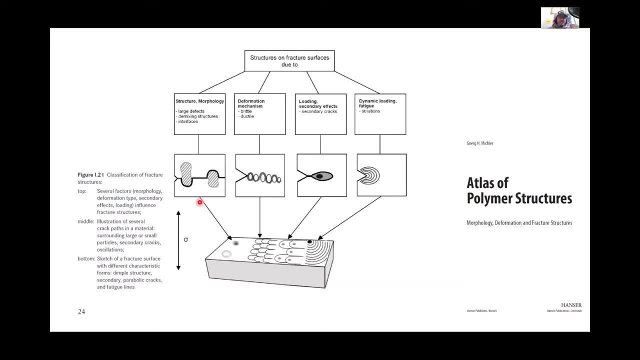 you know demixing structures, interfaces. so demixing structure would mean if you have like a polymer blend and it starts to kind of come apart, um, the interface again, matrix, composite, matrix, filler, interface is what i'm talking about there, uh, deformation mechanism. so if it's brittle, 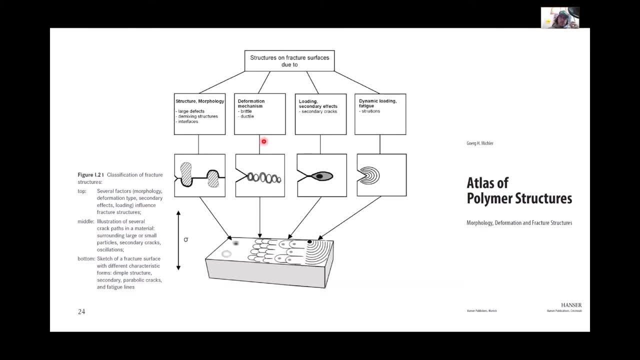 is it ductile? i'll kind of give you a little um kind of preview. if it's brittle, it generally doesn't have that much plastic deformation visible on the fracture surface. if it's ductile, there are- there is- a large amount of plastic deformation secondary cracks. so if it's a loaded, 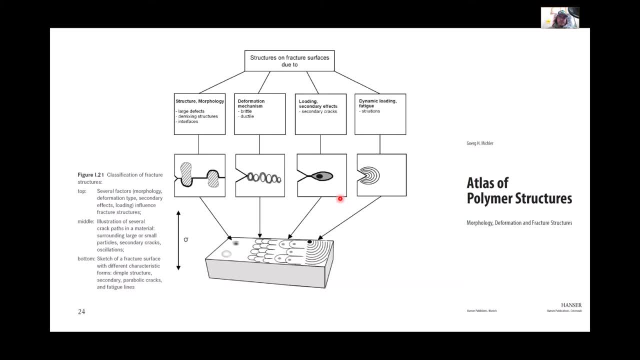 type of structure you can also get like secondary cracks. you also see secondary cracks in a tensile test failure as well. dynamic loading slash fatigue, so you see striations. so we see fatigue striations when we do failure analysis of metal as well and we see that here in polymers. and again i'll show you. 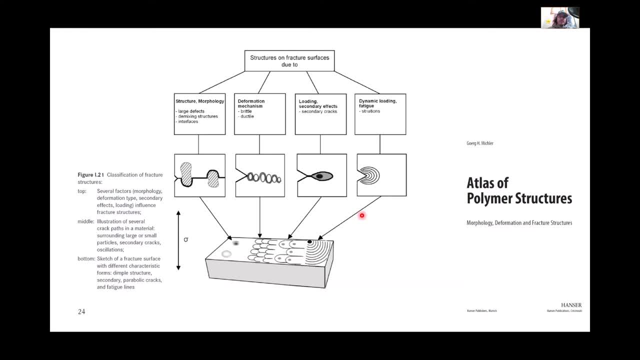 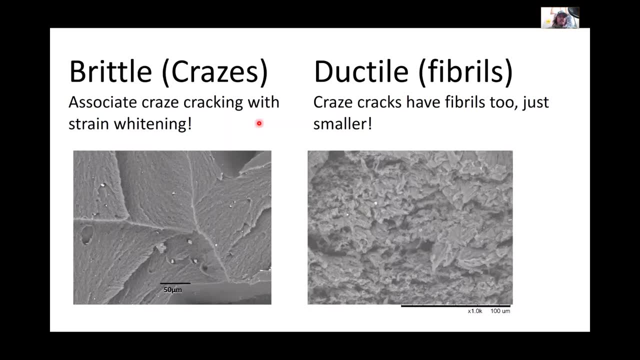 some examples of these fracture morphologies, these fracture surfaces kind of. the first thing i want to kind of harp on a lot is the difference between brittle and ductile failure. we see craze cracking a lot. um, when we have a brittle failure- and i would almost call this one a little bit of a- 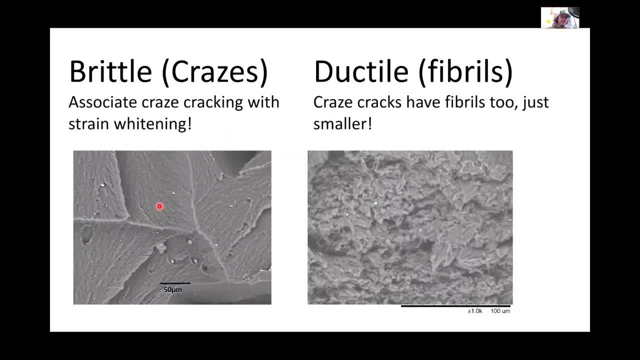 mixed mode failure. this is abs, a fracture surface of abs- acrylonitrile butanine styrene, the same material that legos are made out of- and you see these kind of ridges. these are opened up, craze cracks, and we'll see a little bit more of a schematic of craze cracking here in a moment. 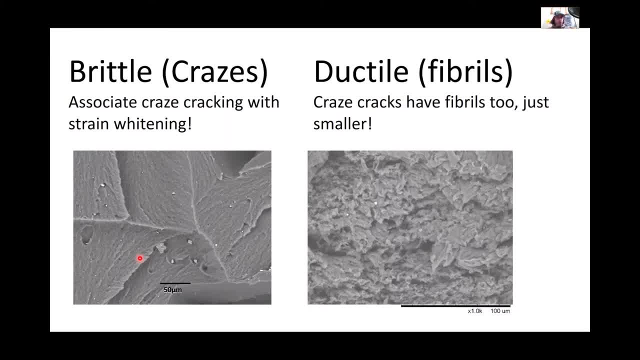 but there's not a whole lot of plastic deformation and i know the scale bar isn't the same between these two. this is actually um well, i have to actually do a little bit of math. it's actually pretty close so, but it's not the same, it's not. 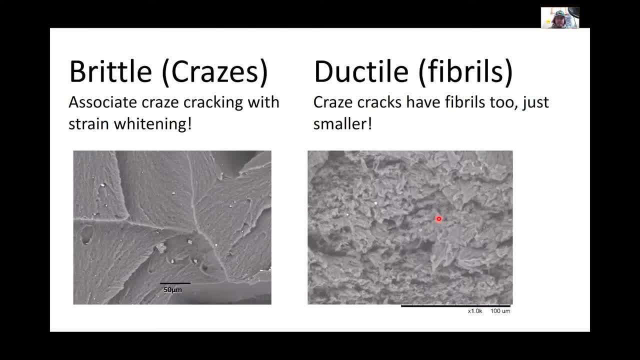 the same scale, but it's not really that far off either. it's not an order of magnitude difference. this is a rubberized blend and you see there's a lot more plastic deformation here, on uh, on this one that i'm kind of highlighting with my laser pointer, and you see these kind of structures. they 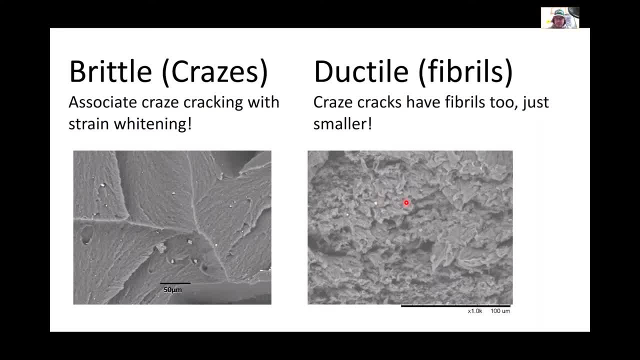 almost look like gum or something. i, i almost, i almost need to find a better descriptor. but you see these, this is fibrils. and the thing i need to kind of point out is that craze cracks have fibrils too. they're just smaller when you see fibril fibrillation on this kind of grander scale. 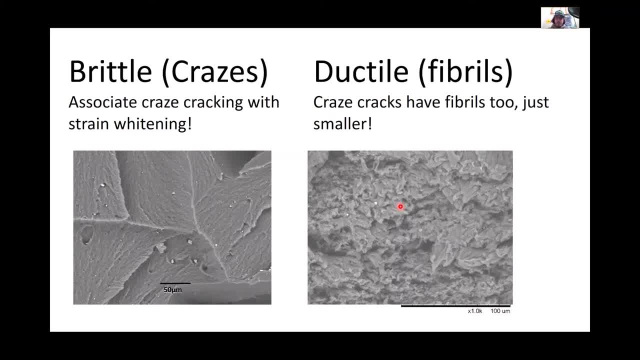 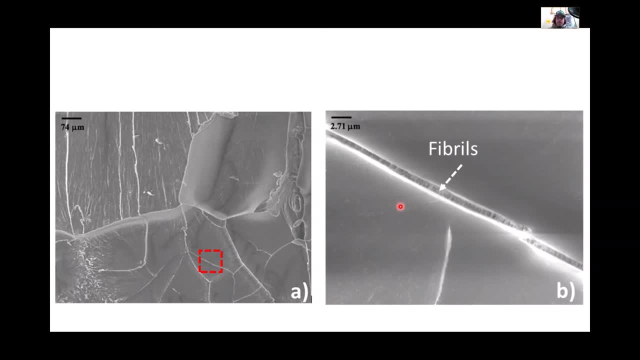 that's, that's associated with um, a large amount of plastic deformation, and we generally associate a fibril, heavy uh um fracture surface with a ductile failure, and here's kind of another example. so this is in a really brittle material, um you can see it's a lot smoother of a fracture surface. um again, you know not. 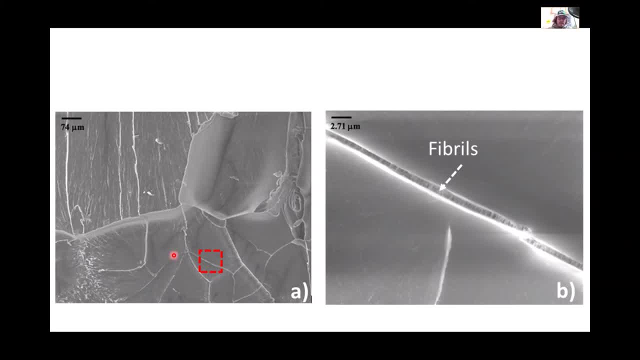 necessarily the same mag, um, but um, we see this crack here, and so this would be like a secondary crack, because the um, what we're looking at parallel to the screen, is the actual fracture surface, but we see craze cracks going into the screen and those would be secondary cracks. and within these, 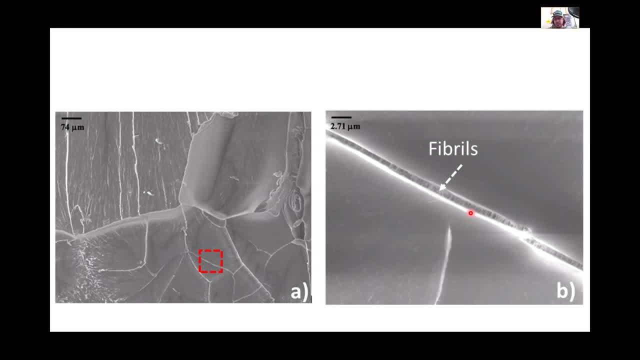 secondary cracks. you see fibrils, and i wish it was a little bit higher magnification, because you can kind of see that the fibrils kind of have a repeating unit to them as well, which is kind of cool because the material is being drawn and and stressed and, um, the material is holding on for 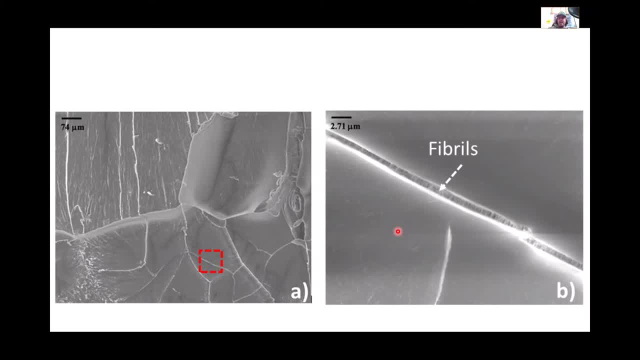 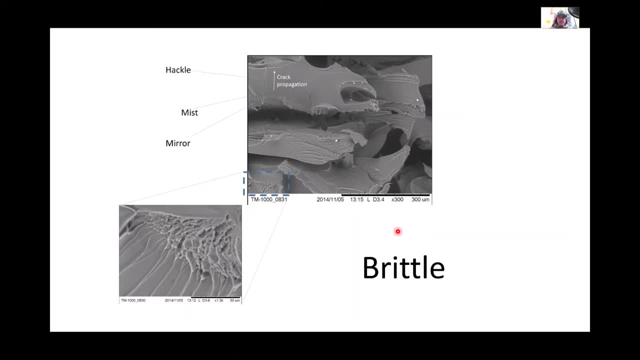 dear life. so your polymer chains are actually a long period of time, so you're going to be able to elongating, and that's what the formation of a fibril is, and I kind of alluded to that earlier in this lecture. when we see a brittle fracture surface, this is kind of a classic brittle fracture. 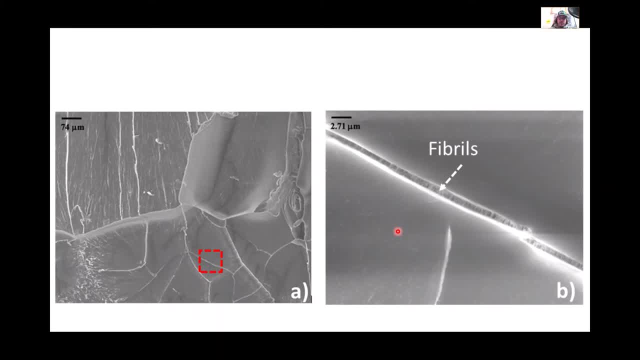 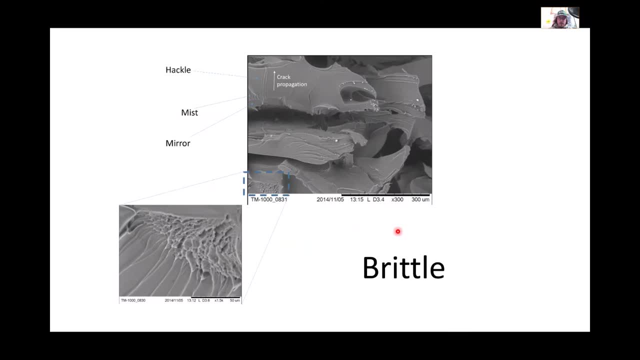 surface. so this is polycarbonate, this material here. I don't quite remember what it is actually. I'm pretty sure this is also polycarbonate, but from a different project. but we kind of see these kind of classical structures and you see this on ceramic failures as well, the so-called mirror mist. 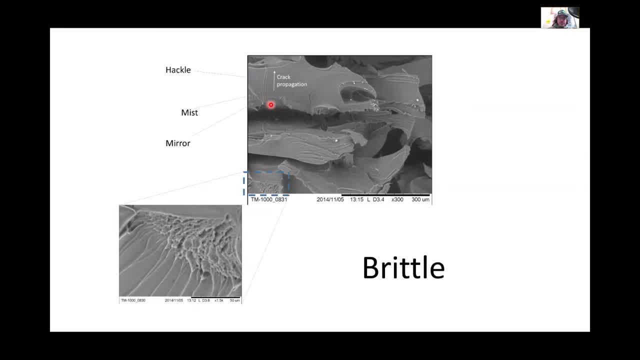 zone. so the mirror zone is generally pretty, um smooth. you have this mist region which I've kind of highlighted in another mystery region here and which looks uh, in some ways. a lot of times it looks like mist, like you sprayed mist onto a mirror or something, and then you have the hackle and these: 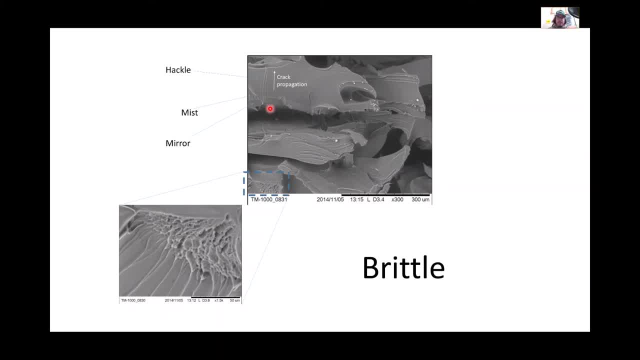 marks are hackle marks and they kind of tell you knowing the relation of these kind of tells you where the crack grew from. and this is a 3D printed structure, an additively manufactured structure, FDM type process, and I'll show kind of a lot of FDM type processes, our images from FDM fabricated. 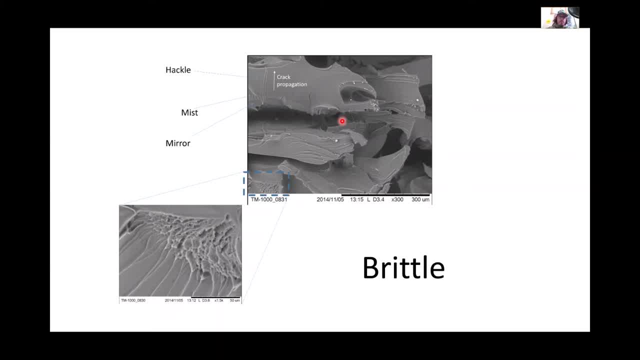 materials in this lecture as well- but mirror mist and hackle- generally fracture characteristics that we associate with a brittle fracture- and it looks like there was a lot of plastic deformation at first glance, but really when you look these are just defects from the printing. so we didn't do. 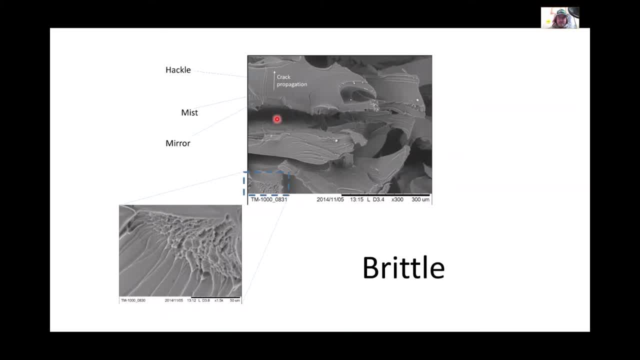 that good of a job printing this, and so this is kind of what we're going to be looking at in this one. this is one raster layer and I don't quite remember what the pattern is, but this is one raster layer, another raster layer and you see there's fracture Services. um crack propagation. 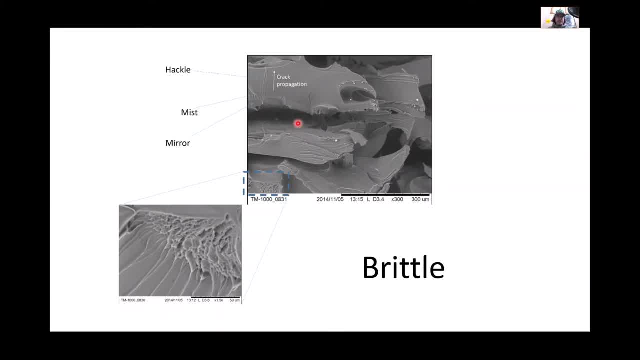 zones, if you will, on each raster layer. so it's kind of cool actually if you think about it that way, because this one propagated this way. we have a mirror zone, we have a mist region and then we see the hackle marks. so we know this one propagated this way. so it's propagating mirror mist tackle. 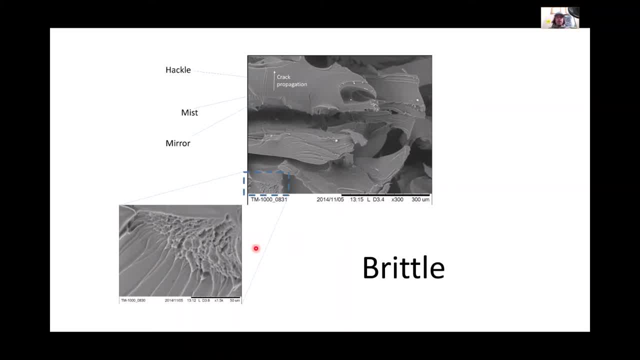 mirror, mist, hackle, in that order. so kind of keep that in mind. so 3D printing structure, different fracture Services, but we're seeing cracks that are propagated in many different directions. it's really kind of a cool thing. I I look at these um quite often and quite happy when I do. I'm kind of. 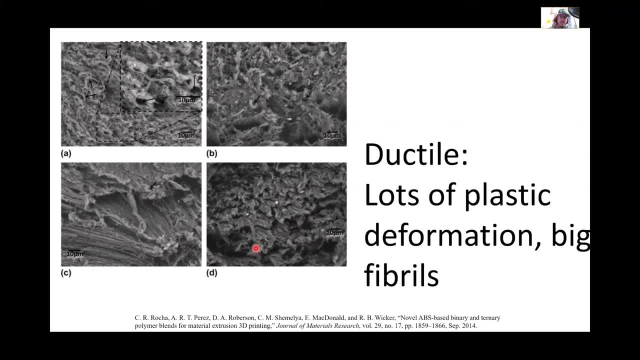 looking um again at a ductile um failure. and this is: these are rubberized uh blends, basically. so I I expect them to be ductile. right, you associate a rubber band, something stretchy, that's pretty ductile and um, anywho, so you can really see, and I kind of tried in the figure and I'm looking back, I look. 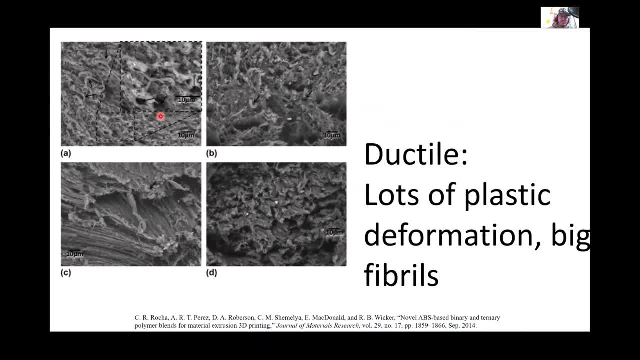 back at my old article. sometimes I'm I'm almost disappointed with myself sometimes, because I probably should have used white as a color here to highlight it a little bit. probably would have stood out a little better. and if you look really closely you see these black arrows and the black. 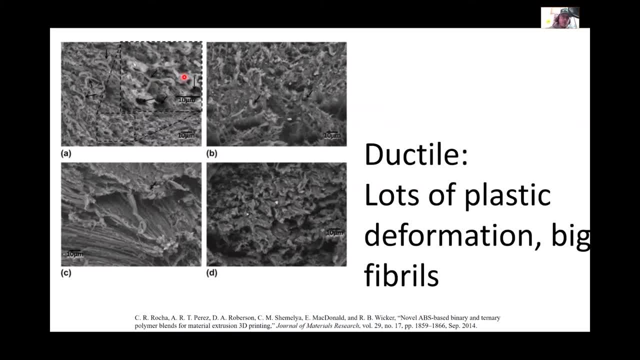 arrows are pointing at fibrils, basically, and then there's a blown up region of this area here, so try to get a better view of the fibrils. this was off that old Hitachi tabletop TEM, not at TM SEM. excuse me, so not the best instrument, but not the worst. 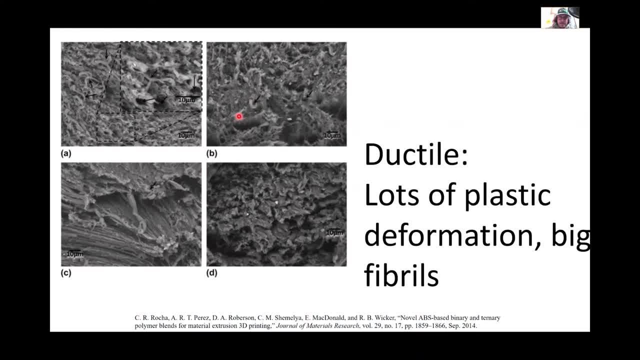 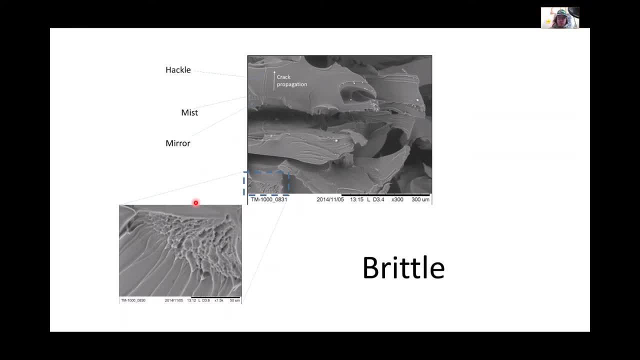 instrument? um, either, but anyway, fibrils. look at that. very nice, ductile, lots of plastic deformation, big fibrils. this is brittle, not very much plastic deformation, to the point where you even see mirror, mist and hackle and we really associate these fracture surfaces with, like glass or another ceramic, that kind of thing. 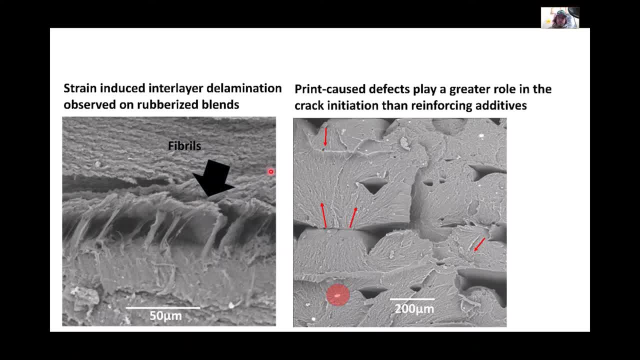 um, here's kind of another example. so we're kind of we're comparing a ductile brittle. these are both 3D printed structures. this is one, uh, one layer and another layer, and the layers actually stuck together pretty well. so we have kind of this strain induced delamination and so we're 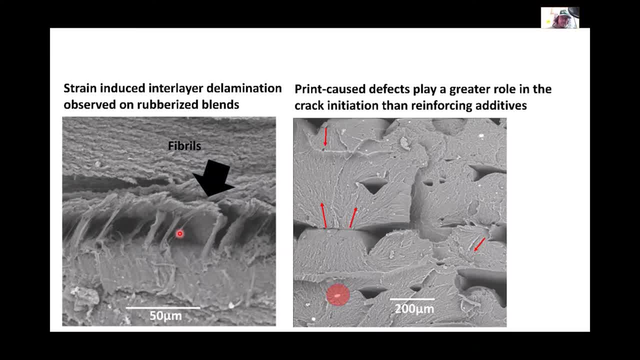 kind of seeing these fibrils holding them together. so that's actually kind of cool. this is an actually a ceramic loaded polymer and we're kind of seeing that the inner layer defects are actually playing a bigger role in the failure of um, of this um structure, this test specimen, if 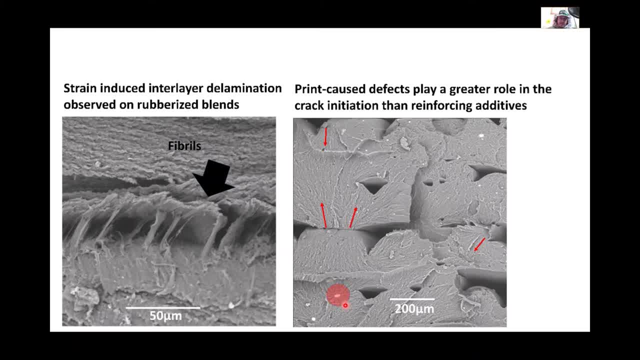 you will, than the reinforcing element. so I don't see that big a sign that this filler material would play that much of a role in the failure of of this, as compared to what I see in terms of the inner layer defects. here's an example of where we know our additive. 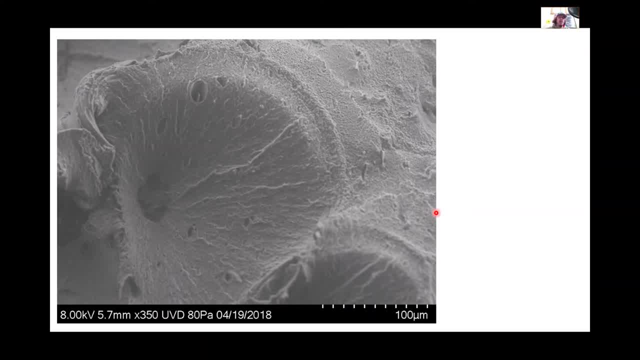 uh was causing or actually contributing greatly to the failure. this was a bad attempt actually by me to incorporate graphene oxide into a material and you kind of see, and there's actually a bit of associated with this. but anytime you see something circular on a fracture surface like this, this is a strain field and the particle here, this geo particle, we 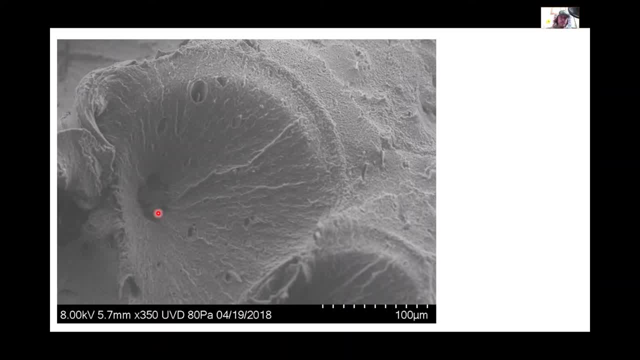 agglomerated, basically agglomerated- graphene oxide led to a stress concentration to the point where actually formed a stress field and you see kind of these secondary stress fields even forming here and they're generally spherical. so if I hadn't opened this it would be pretty spherical. 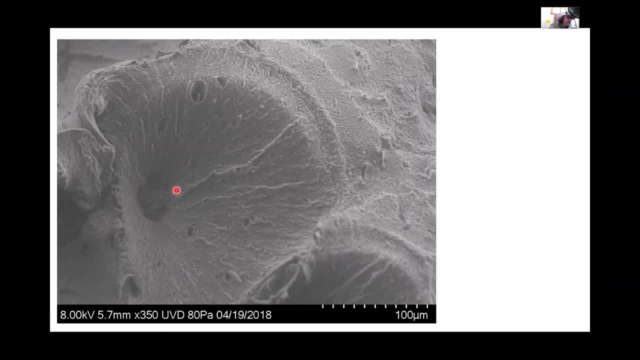 if you've ever taken likes like scotch tape, cellophane tape, and then kind of put it down and pilled it off and looked, you kind of see almost like circles on it. so try that. I should probably try it on camera here and maybe I will try to. 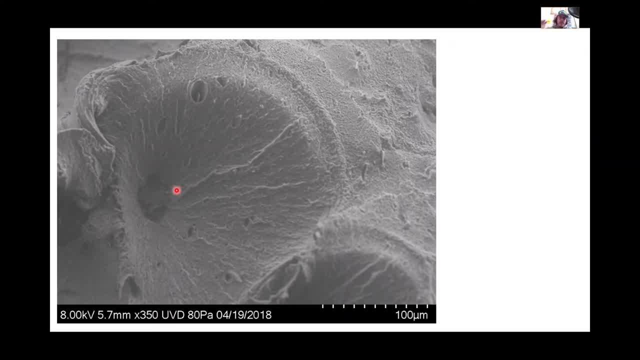 throw it in, if not. you know, I failed in my home experiment because I'm putting it here and then I'm going to try it on camera and maybe I will try to throw it here on video, but strain filled, so kind of. keep that in mind too. this is another. 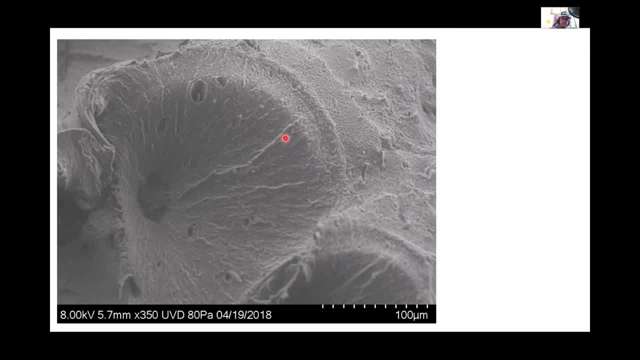 fracture surface feature that you kind of want to play in mind. it's really kind of cool. I'm really neat. you kind of see the manifestation energy was trying to be lowered. you made, made something spherical and you even see it here. there's something else kind of sticking out here, but you almost see kind of this. 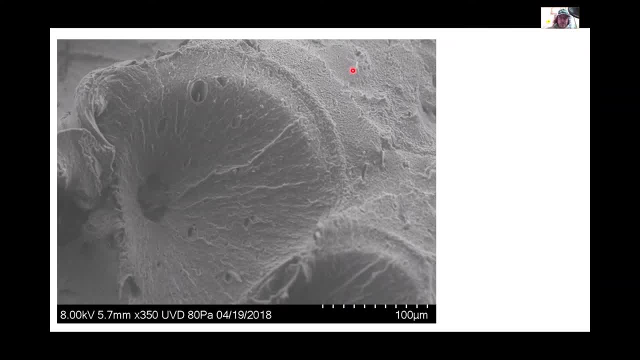 spherical structure or circular structure around it and don't see much plastic deformation here. so I would kind of say this is maybe. well, this looks pretty plasticky. so I would kind of say this is a mixed mode ductile brittle fracture, but it was generally definitely aided by, in fact, 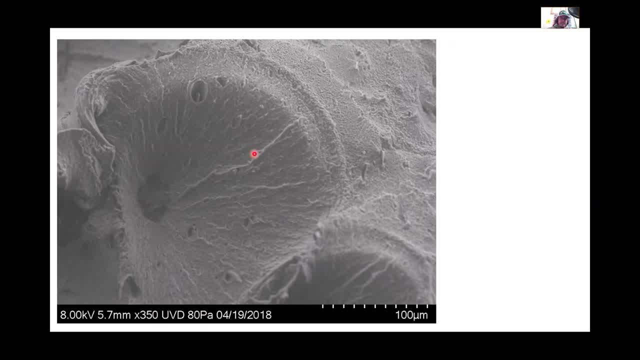 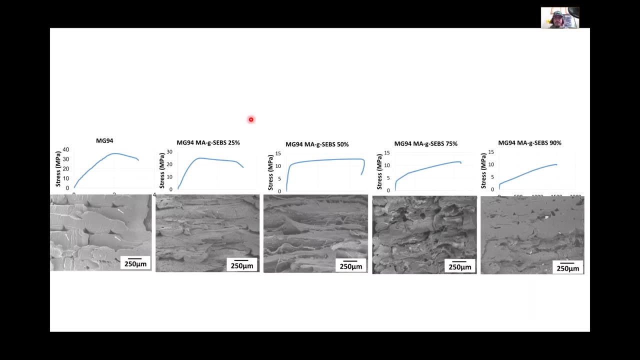 we see two kind of intersecting stress builds here and they're due to the stress concentration of this filler material. so we didn't do a good job making this composite. I'm kind of showing the effect of adding rubber and I've shown this before and it's uh, I'm missing the source this time. I 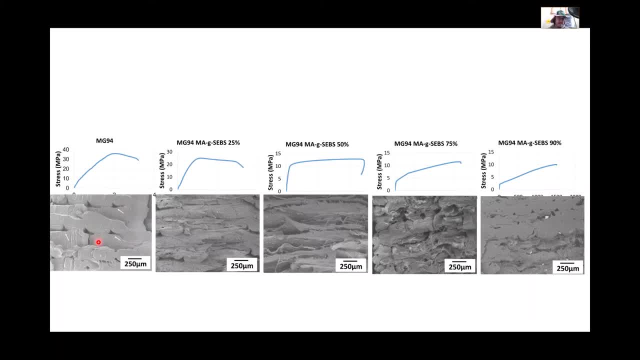 apologize, but this is just ABS, and so we kind of see this kind of brittle mode failure when we start adding rubber to it. so this is a maleic and hydride grafted sebs. we start adding rubber to it at different levels we see an increased amount of a plastic deformation, but then we get 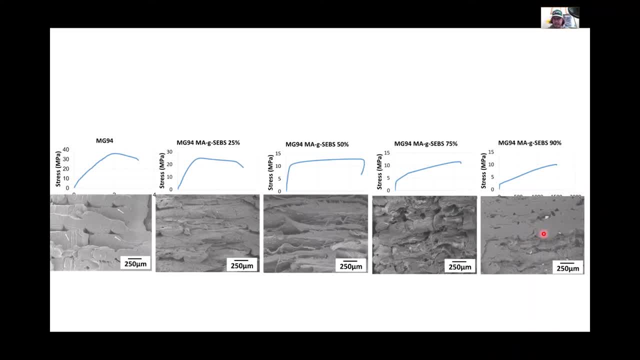 here and it doesn't quite look like there's as much plastic deformation going on, and we even see those look like strain fields there too, which is our stress fields, excuse me too, and uh. so what's going on here is actually kind of interesting, and I kind of messed up the figure a little bit. 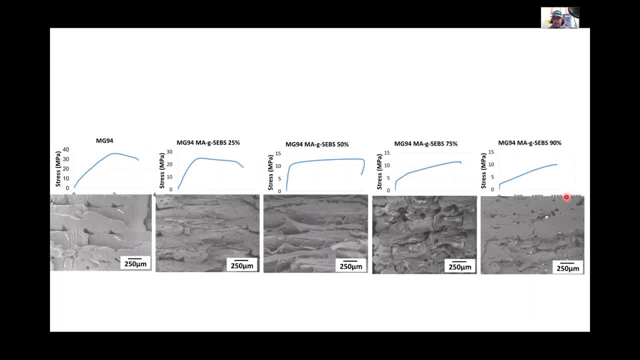 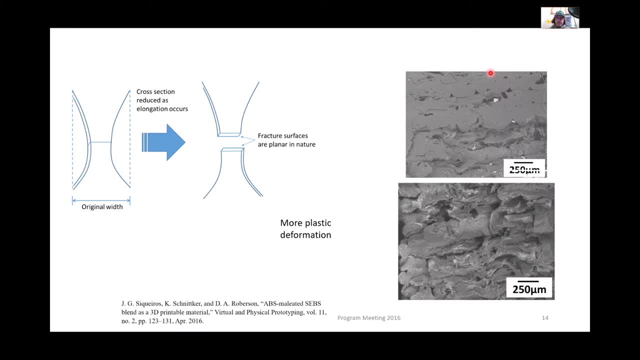 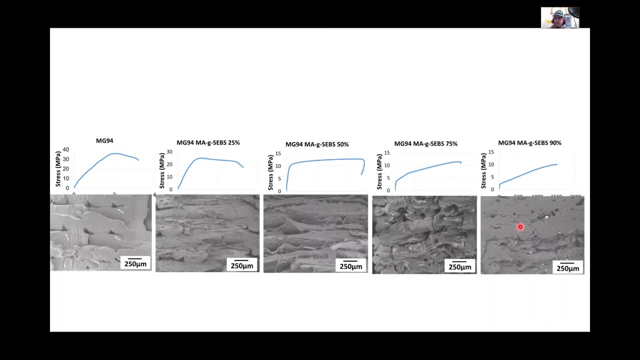 because I don't have my scale, but we're uh, 1500. elongation is this one, so it elongated quite a bit. so that hopefully gives a clue to what actually happened. so for this heavily loaded um sebs material, material or heavily rubberized material, in fact it was 90 rubber. basically we necked it so much. 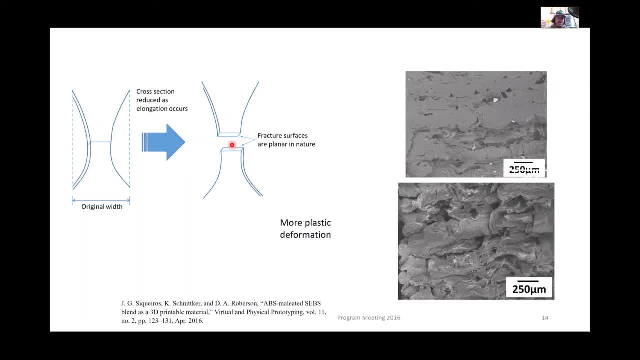 and so the uh. what basically happened was the cross section was affection. it was effectively reduced and, um, you ended up with more of a planar fracture surface. so you don't really appreciate the plastic deformation that occurred before this material ruptured, and so always kind of be aware um that that uh, sometimes it may look like a brittle failure, but 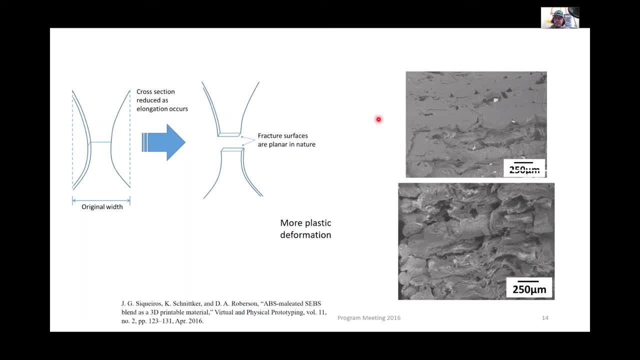 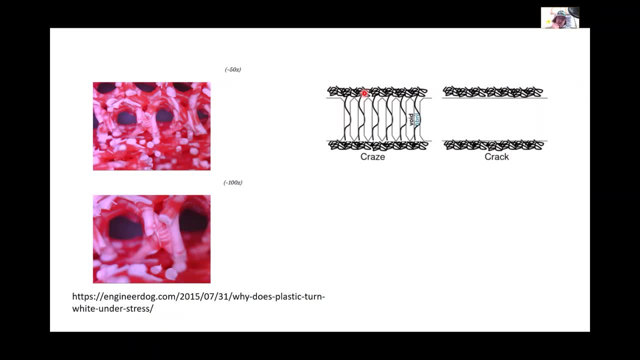 it was really a very, very ductile material and so kind of interesting. I made some mistakes here on this slide trying to figure that out. looking, uh, here I got this from engineering dog or engineer dog I tried to make my own pictures of of stress whitening and I really just couldn't. 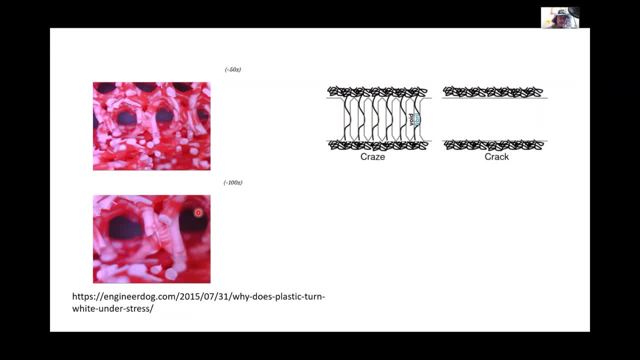 uh, these, this is a 3D printed structure actually, and so it was kind of fitting, because I tend to talk about 3D printed structures quite a bit when I talk about failure analysis and composites and stuff like that, because I do a lot of that myself and you see, here it was a red material and it was. 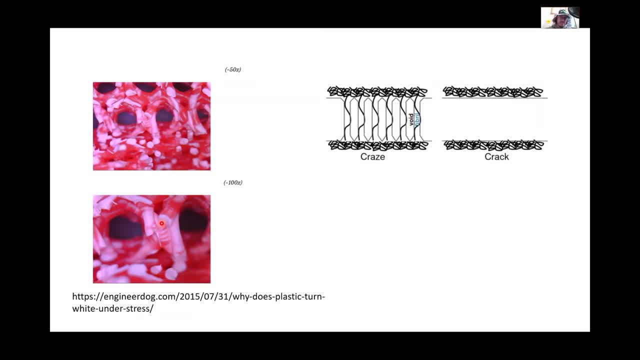 a broken and it wasn't a tensile test specimen. it was like a disc that they broke and you can, if you're interested, you can kind of look at this URL, um, but this is um. strain whitening basically is what this is called, and this course actually exists because of strain whitening and there's 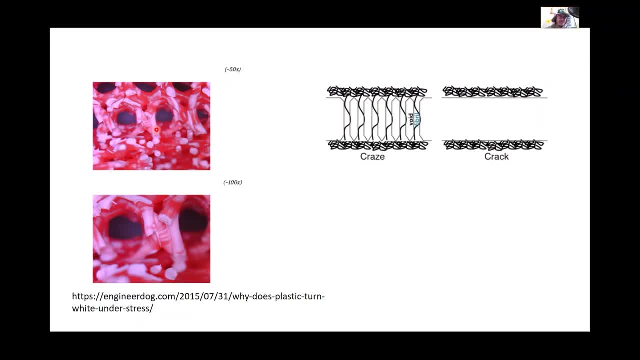 kind of a longer story associated with that. I may tell you somebody at another time. but anyway, strain whitening associated with craze cracking. again, here's kind of a schematic of kind of the craze formation and then you, it actually ruptures, so these chains will eventually break. there is 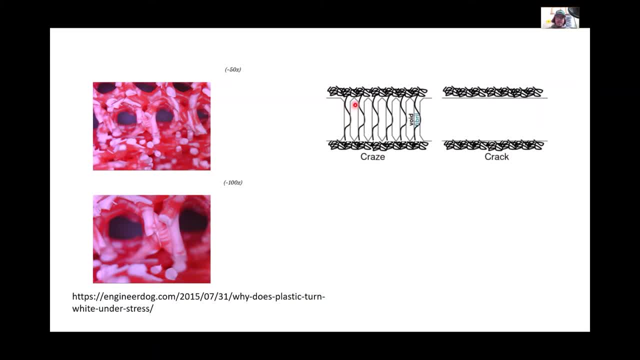 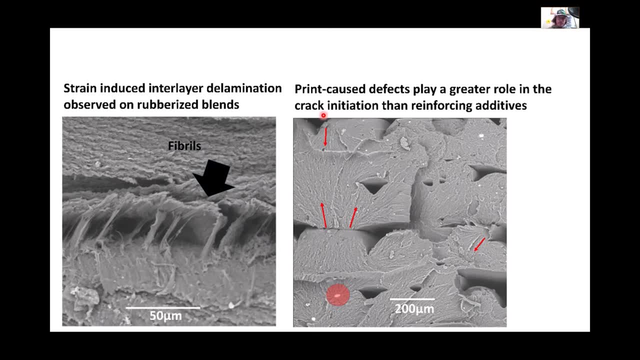 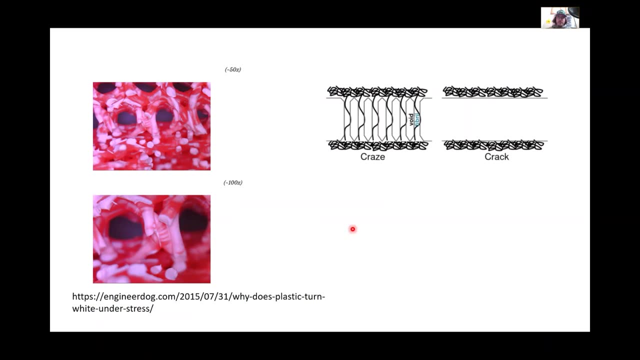 some elongation going on of the polymer chain. so you get these micro, micro fibrils, if you will. these bigger fibrils, I tend to refer to them as macro fibrils. they're a little bit bigger than something on, on almost a molecular level really, because it's an individual polymer chain that's stretching out craze cracks. a whole bunch happen. 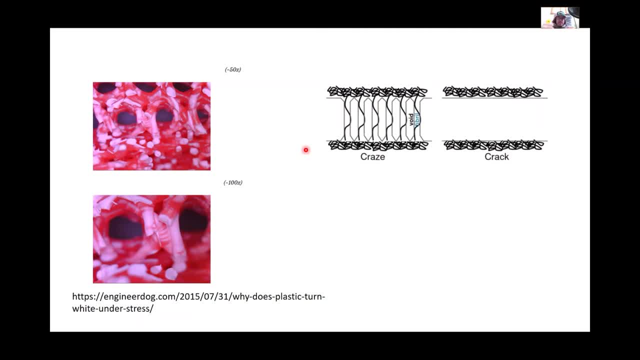 in kind of the stress zone, if you will, and eventually a final rupture occurs, and but it was cracking all over the place before the final rupture occurred, basically, and so this whitening is a craze crack formation, so strain whitening fibrils. this was answering the question. why does plastic turn white under stress? 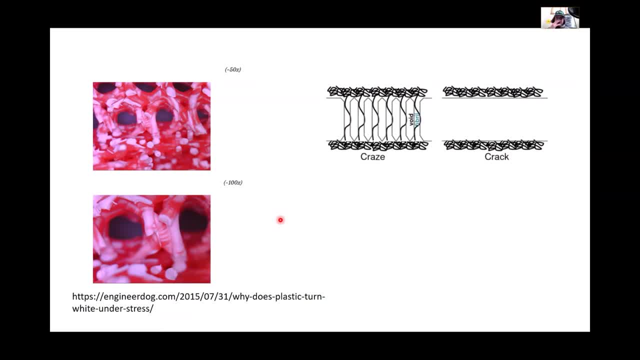 okay and so, uh, it was very fitting, so I borrowed it from this. uh, this website couldn't make a good picture of my own, unfortunately, but again, anytime you look at polymer and you can actually take a plastic spoon- probably a black one- would be better to see it. 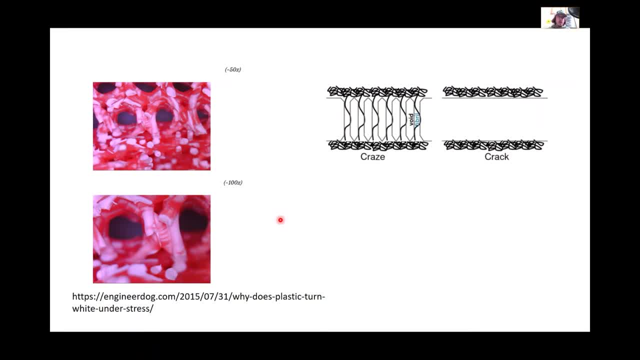 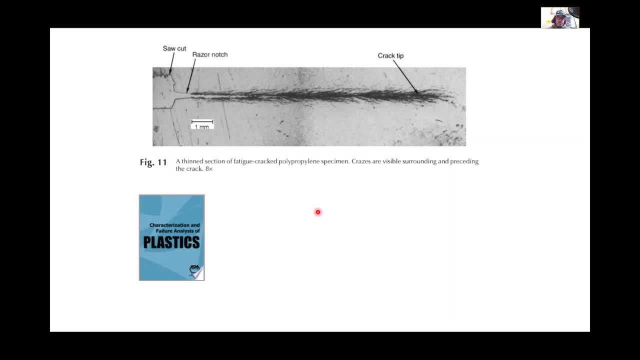 and if, when you see that whitening occur, that's that's strain whitening and it's the formation of craze cracks. here's another kind of really cool- excuse me, um, really cool, um, I guess- depiction of kind of craze cracks propagating through and it kind of shows this crack tip propagation kind of. 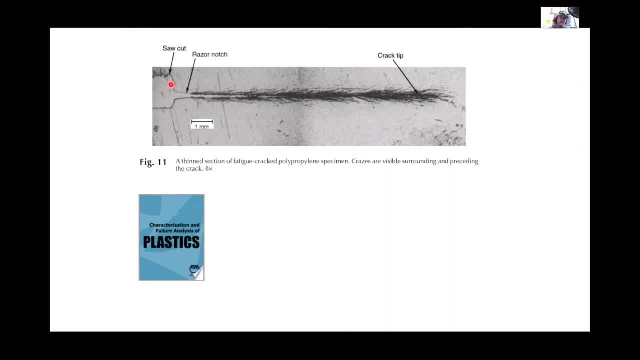 moves through the material. this was a result of a kind of a double stress concentrator, right, so they saw cut, then they put they call it a razor notch. I guess they cut it again and the crack propagates through the material based on this stress concentrator, and you kind of see these craze. 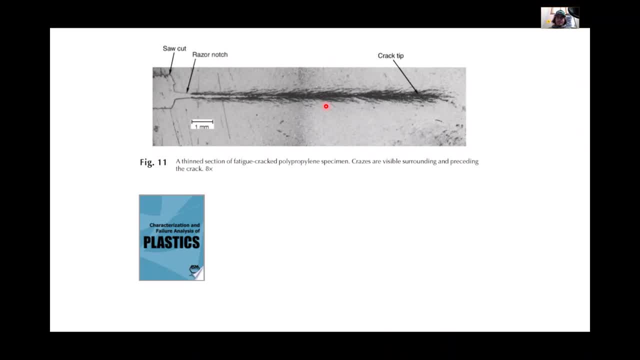 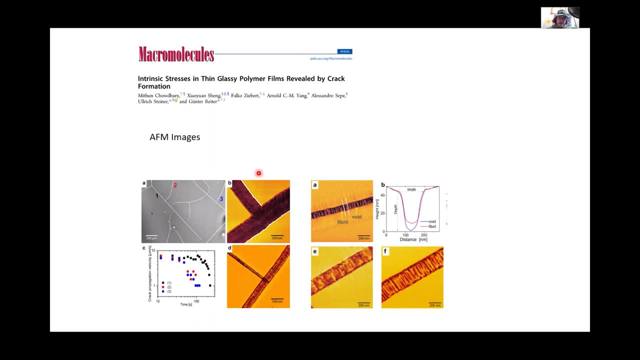 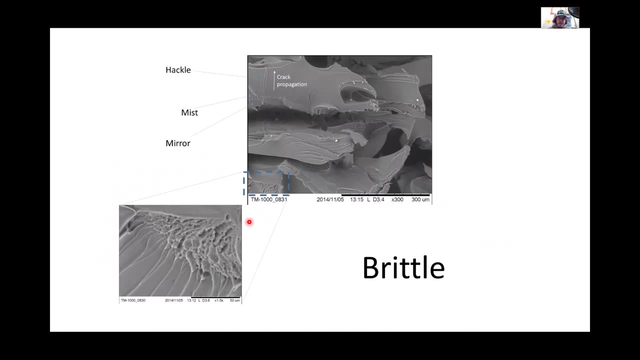 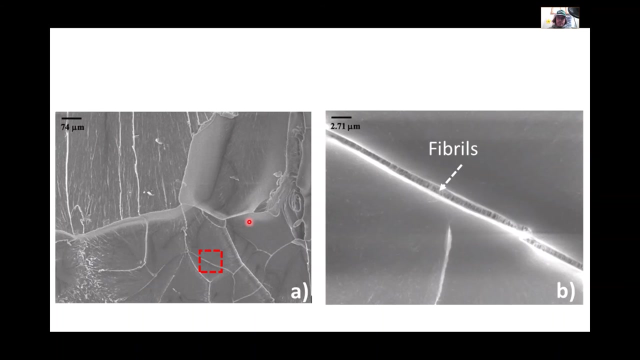 cracks. this is really really kind of cool. I like craze cracks. if you haven't figured it out, here's another example of craze cracks, and this is very similar to the figure I showed up here, and so this one came out of our lab and we've yet to publish this work. we're actually in progress, so maybe in later years when I show. 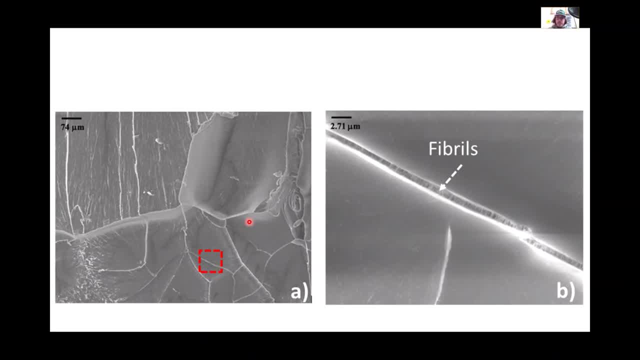 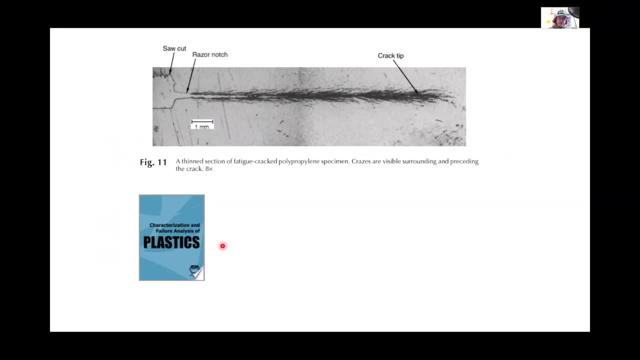 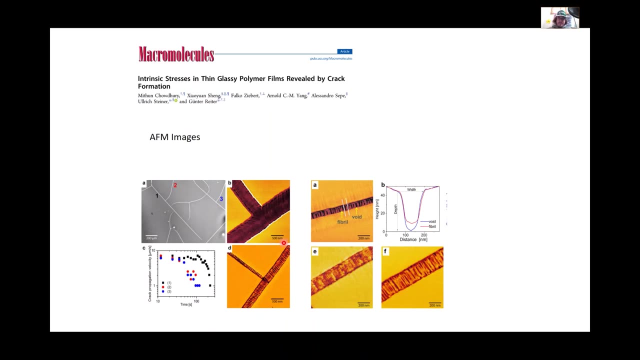 this video. again it'll be a published paper but anyway. so we see fibrils. I'm living in the crack and see it again in this other individual's article, in a- excuse me, this article here, excuse me, I threw myself off- and again you kind of see the fibrils form with a, with a fairly regular 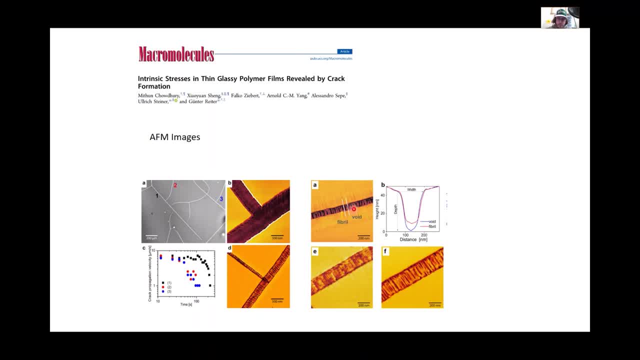 thing, and so fibril void. here I have to interpret the contrast, but it's telling me. so the the darker spots, the void, and really really cool. um, they apparently use atomic force microscopy to see their fibrils and this is an sem image and this is. these are AFM images of um, of the fibrils I'm. 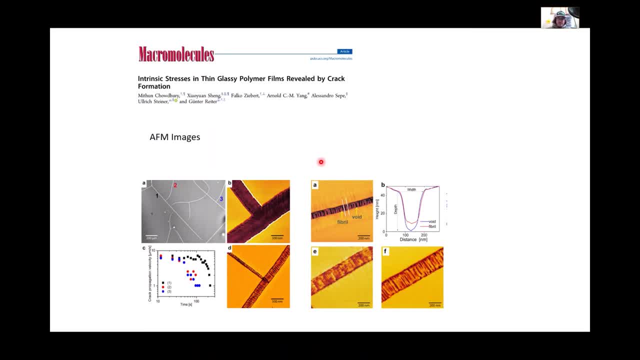 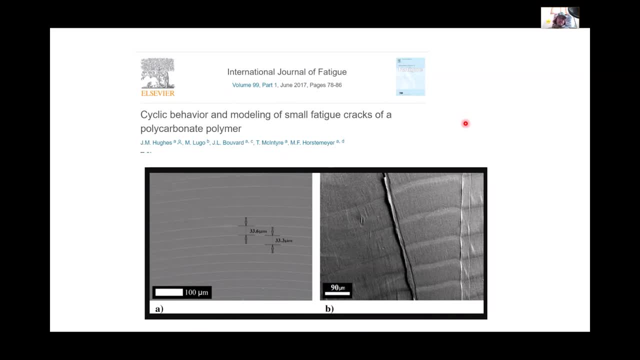 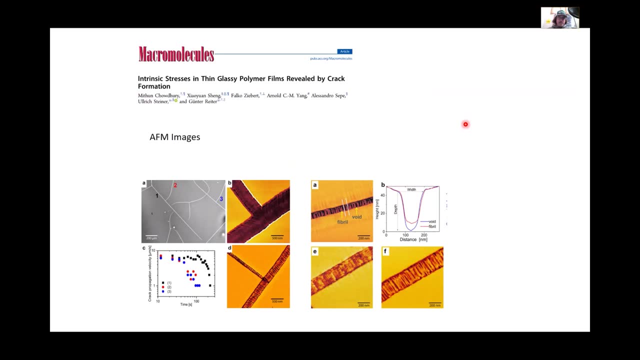 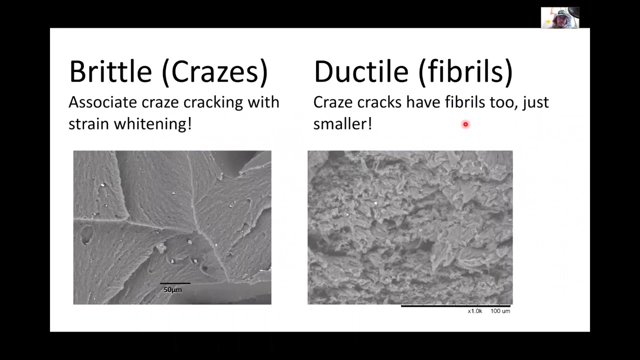 sorry of the um yeah, fibrils within the craze cracks, basically. so it's. it's kind of cool, um, looking at a cyclic failure. so earlier in the lecture I kind of showed examples of different polymer morphologies. I've harped a lot on ductile brittle and let's see what other kind of preview. 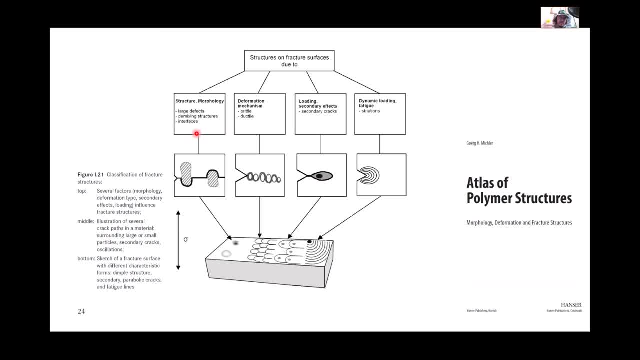 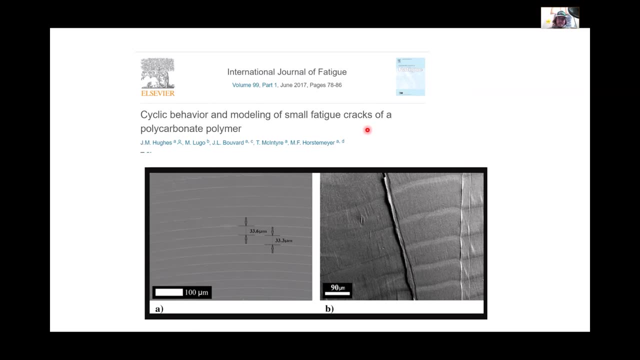 um demixing structures, interfaces. so we've seen interfaces, we've seen ductile brittle and we've even seen secondary cracks, and now we're going to kind of look at this dynamic loading situation where we see fatigue striations and these are really nice, actually very evenly spaced, and this 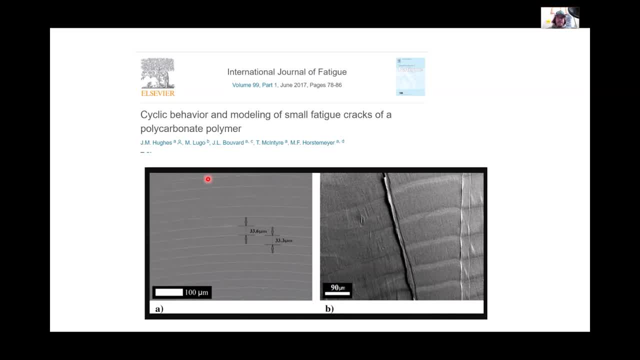 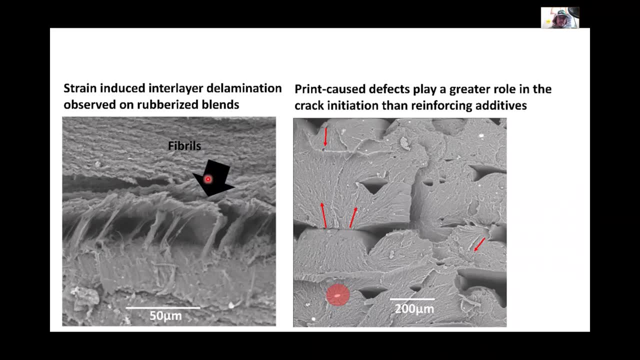 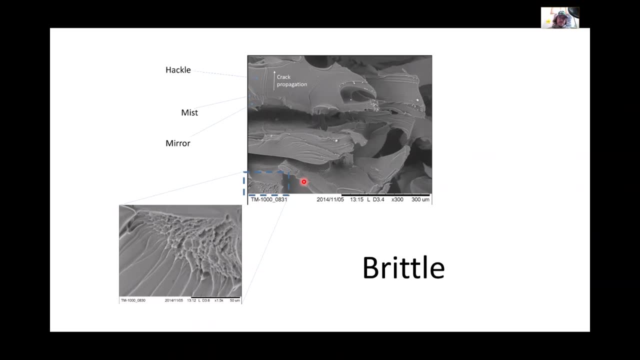 is polycarbonate, which you know actually fails brittle, and so this is a cyclic failure of polycarbonate. if you go back and look at this, where did I show this one? this is not a cyclic failure of polycarbonate. this was an utensil test, so a dog bone, so we're looking at the fracture. 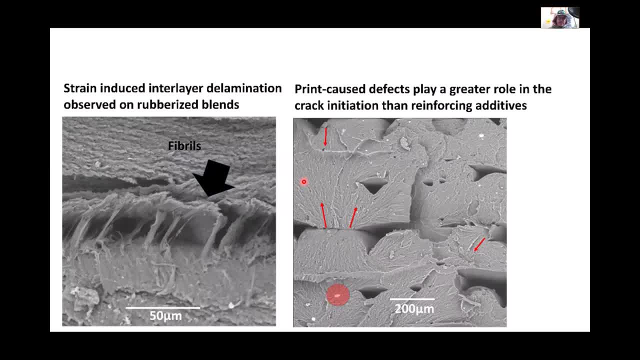 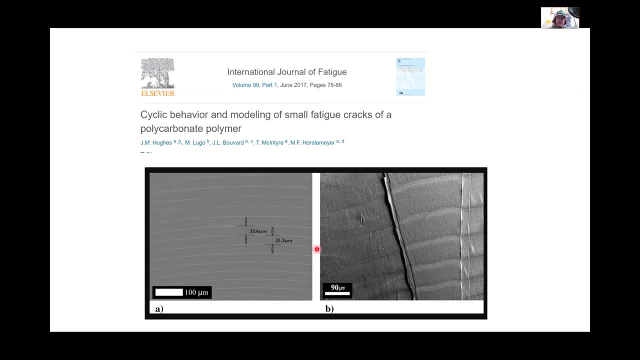 surface of a dog bone text utensil test specimen. this is a fatigue specimen and again you see fatigue striations and you can tell where the crack propagated, very similar to what we see in in metal fatigue. and so the crack propagated this way, or I should probably. 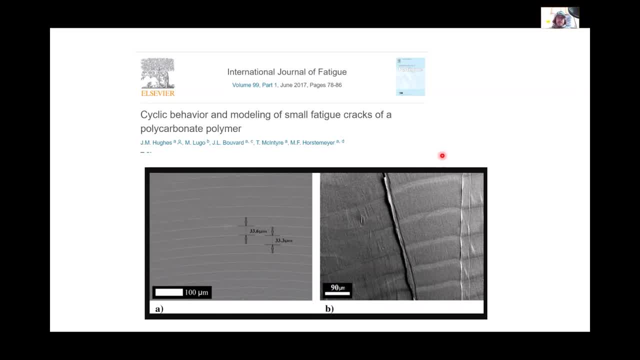 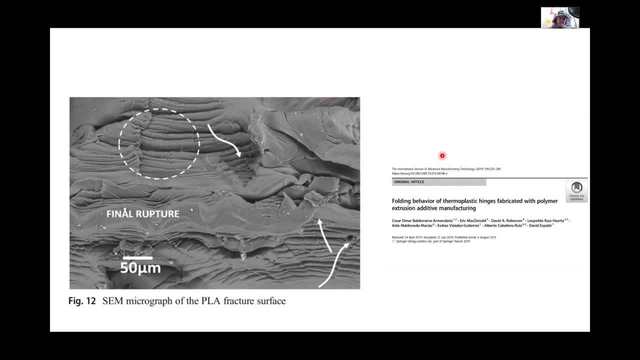 do it with the laser pointer this way and really kind of cool, these are fatigue striations. we kind of did our own experiments as well, where we made these hinges, and this is actually PLA, which isn't the most ductile material, but we still see fatigue striations here. this was a living hinge. 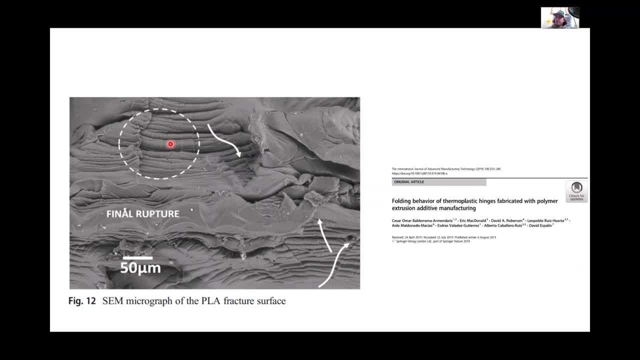 and I've kind of- I've kind of- talked about living hinges before in this class, where it's it's not, you know, a mechanical structure. it's basically like folding a piece of paper and you just use this. it's like folding a piece of paper. so if I fold a piece of plastic, it's a living hinge. 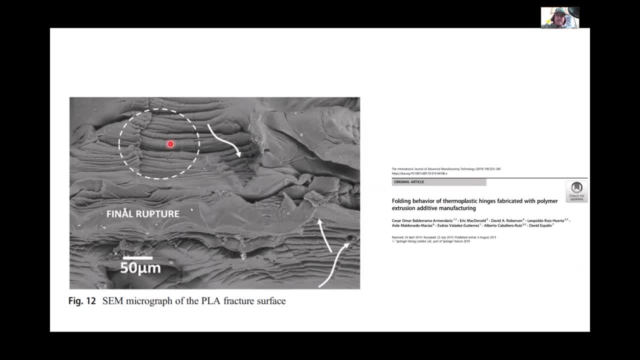 basically, and so again we see these fatigue striations. the final rupture occurred in this, in this case in PLA, in the middle of the uh of, in the middle of the hinge, and so it propagated going this way and it propagated going this way, and again we see it's a little bit different than than these here. 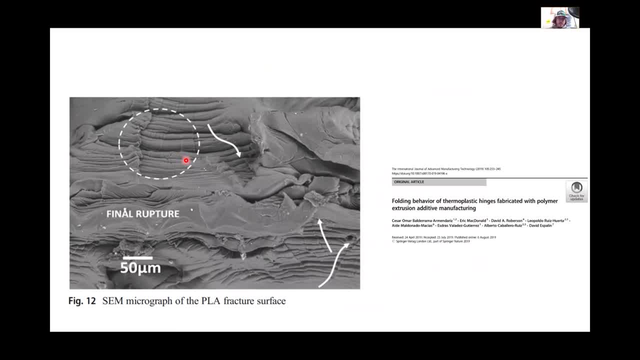 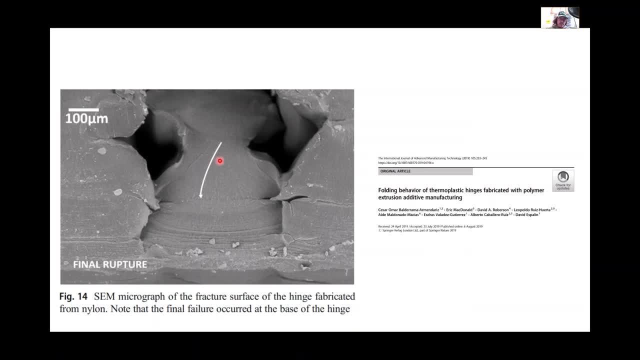 fatigue striations right, a little bit different, but this was a hinge, really kind of cool, um, seeing it again in a different material. so this was nylon, and the failure actually occurred at the bottom of the hinge for this one, and so we only have one crack propagation or crack. 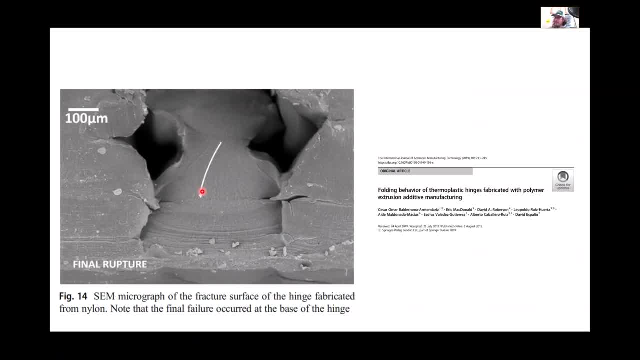 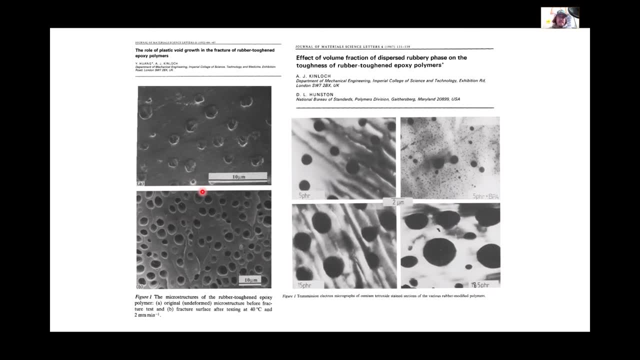 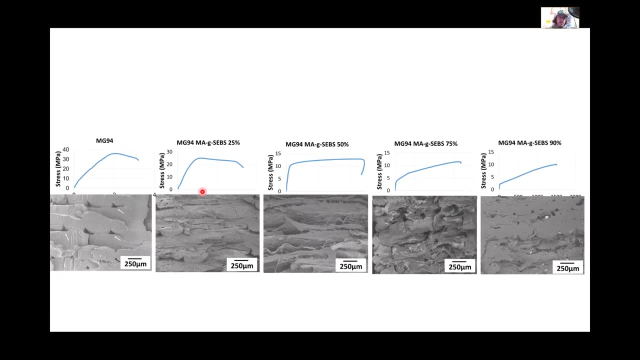 propagation Direction, excuse me, um, adding rubber to material changes things, and so we've seen the effect of adding rubber, uh, to you know, basically the failure mode, if you will, of of ABS, and kind of once you get to the 50 here, right? So these are probably the ones you want to compare a little bit more, And so 25%. 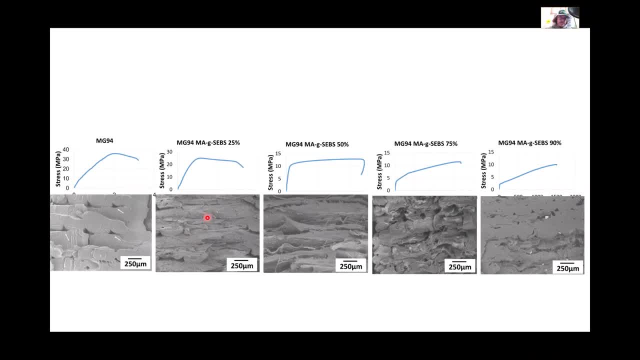 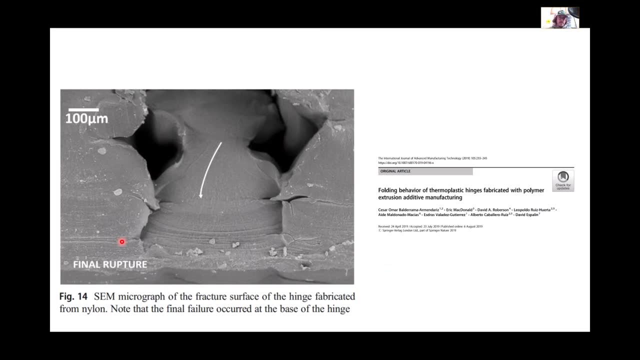 SEBS. very dramatic difference in the fracture surface morphology as we see, compared to just pure ABS And ductile ductile kind of see some brittle Here. this is actually kind of cool. ABS itself actually is rubber toughened. It's a styrene acrylic nitrile with butadiene spheres in. 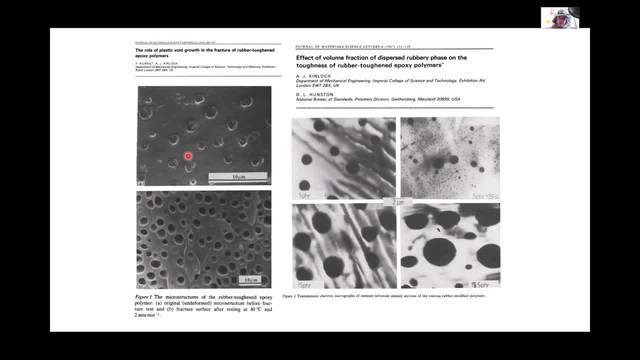 it. But this is kind of showing: they cut it here And so you see they've put these rubber spheres in this epoxy And then when they actually deformed it, you actually see the spheres deformed themselves under a tensile load And again they're dispersing rubber within the 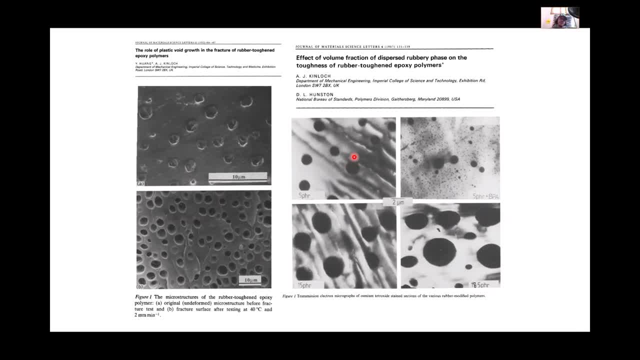 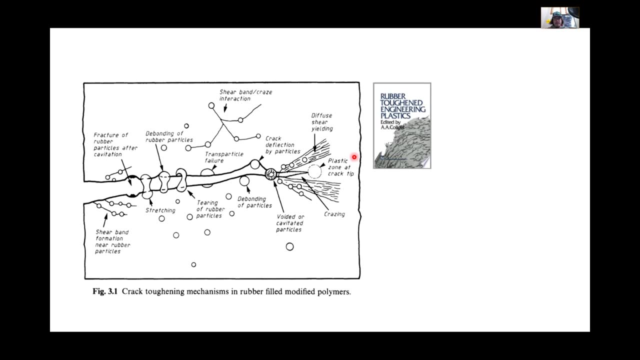 material. So you have kind of this two-phase structure, And rubber generally leads to a toughening, So it's rubber- toughening is what you tend to call it- which is really happening now And you could kind of say this is a reason why the fibrils are bigger, But you have these rubber particles. 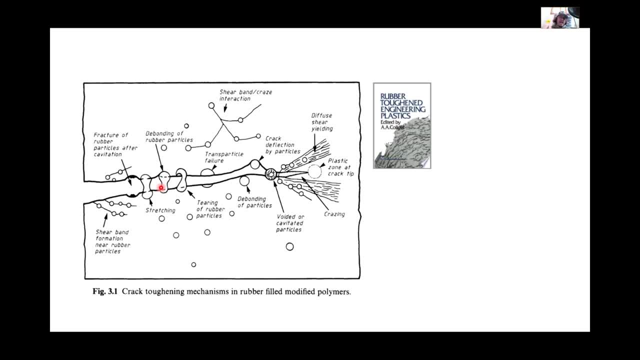 and they're kind of arresting the crack right, It's going to eventually fail anyway, And so what ends up stretching is the rubber component of your mixture, whether you have something like dispersed rubber or not, And so it's kind of a reason why the fibrils are bigger, And so you 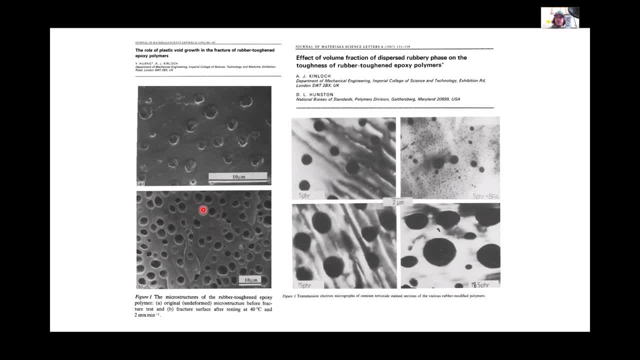 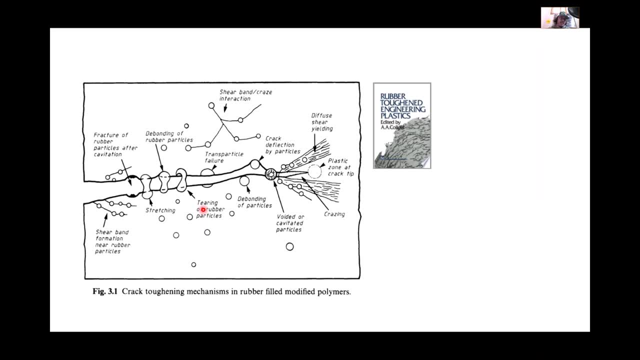 have these rubber spheroids in your material or you have these rubberized blends And I've shown the microstructures in previous lectures. So if you want to kind of see the microstructure of these ABS-SEBS blends, I've shown that in the blends lecture And I am a little remiss for not showing. 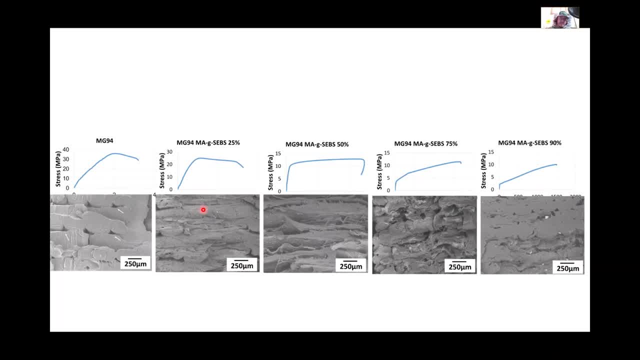 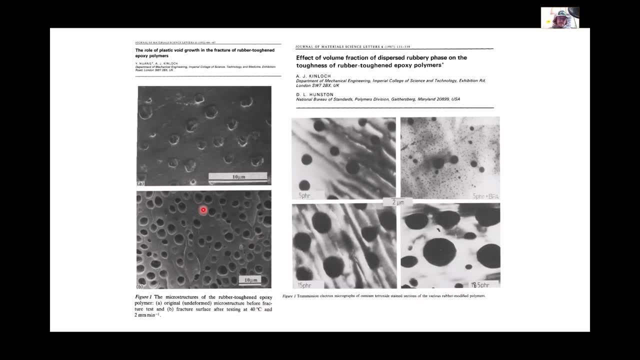 it here, But here it's more of a two-phase system, So it's a little bit different than this type of system, excuse me, this type of system where you have these dispersed spheroids And so it's kind of a two-phase system. So it's a little bit different than this type of. 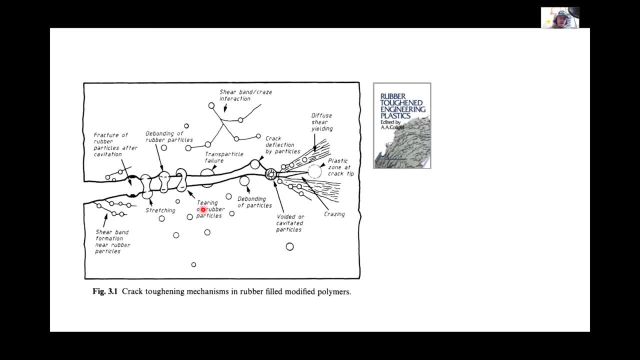 system where you have these dispersed spheroids of rubber. But when you have these dispersed spheroids of rubber they tend to arrest the crack And, instead of the material itself, the individual polymer chains stretching during the formation of crazes, these rubber particles. 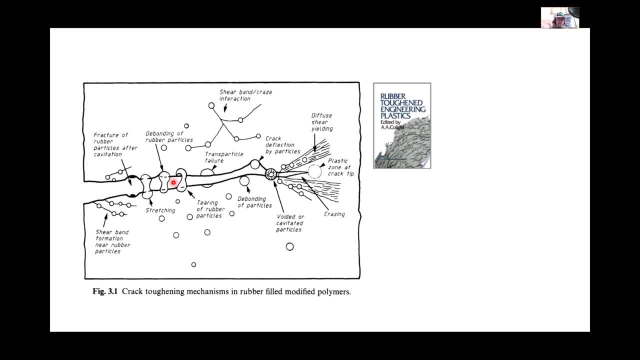 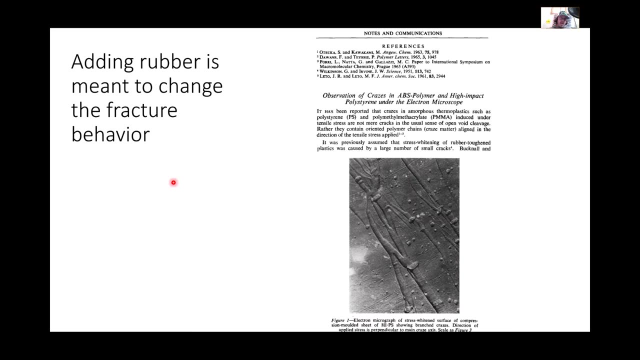 tend to stretch and actually resist the overall failure of your structure, And so that's kind of a mechanism for rubber toughening. It's crack arresting in this case. Okay, Adding rubber basically meant to change the fractured behavior. And this is very old So 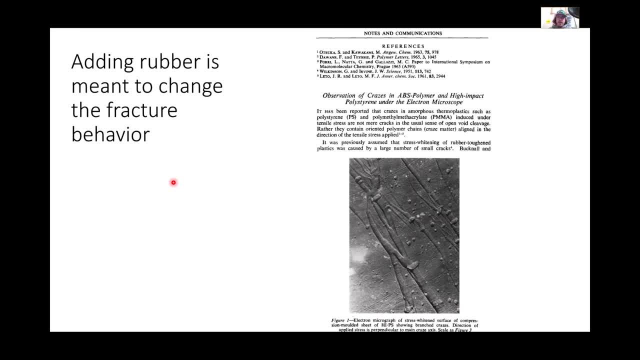 people have been doing this for quite a while. I won't talk too much about that. I don't think it really complements anything else, And it's kind of hard to see because you can't really see the two phases. They didn't do any staining or anything like that, But you kind of see these. 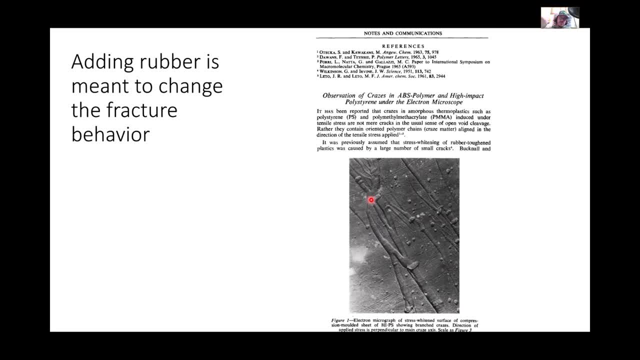 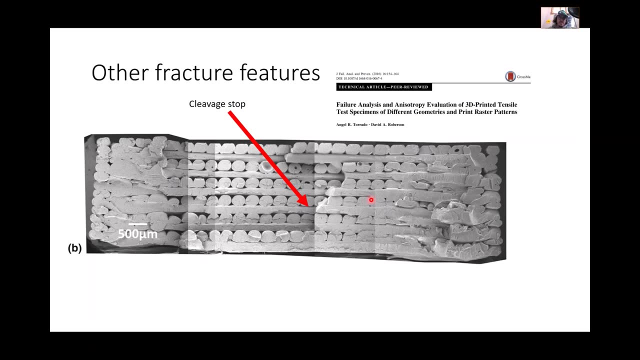 cracks, So it's holding the material together, It's preventing this material from reaching final rupture or delaying final rupture, basically Kind of other fracture features that we tend to see on polymer structures. And again, I kind of did this old school, I did this cut and paste, I did. 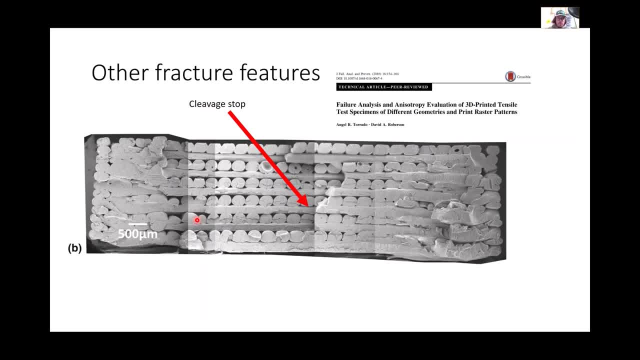 it digitally, But I've been told that there's software that actually would have allowed me to blend the contrast a little better, And so I wrote this with a student, Angel Torado, or Angel Torado, And so I'm taking the blame for 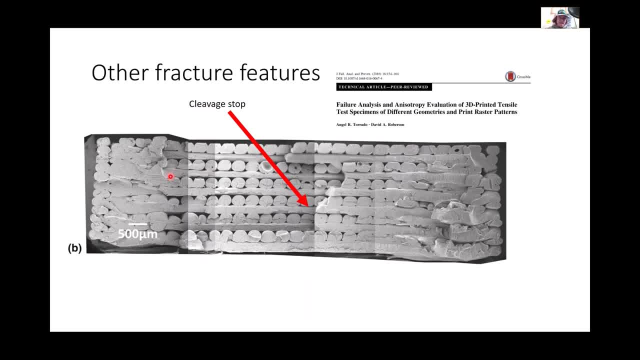 the contrast, because I put these kind of big ones together. But, anywho, when you see- and this is more planar than it looks because of the contrast, but this definitely is a ridge- And when you see, these ridges pop up on fracture surfaces, So here's one, And then here's the other one, And 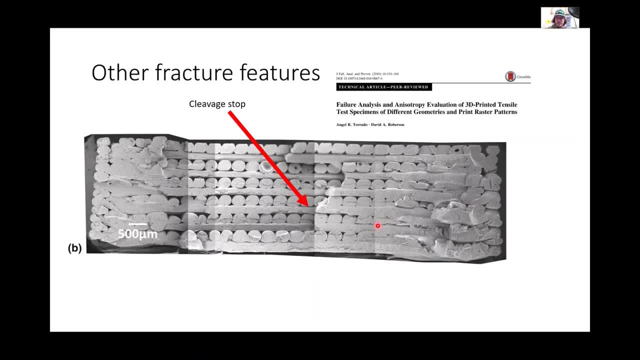 here's another. These are called cleavage stops, And so we kind of see there's a lot of propagation directions here. These are like secondary propagation directions, But the overall direction of the crack propagation was going this way And then it stopped, And then kept going this way And then it. 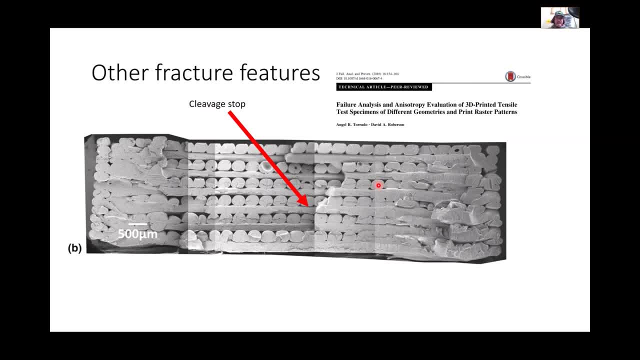 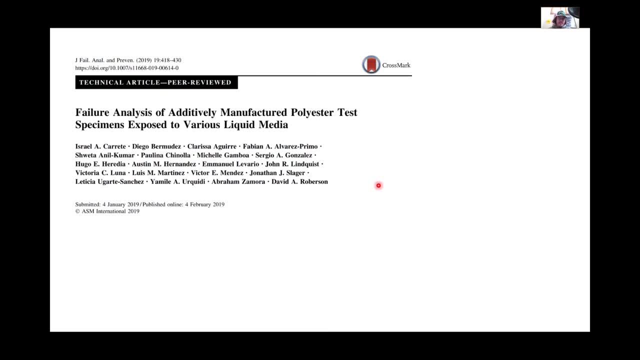 stopped. So these are cleavage stops. So that's a fracture surface feature. I want to kind of draw your attention to that. So cleavage is come from this article that we put out, And so what we did was we took two polyesters. 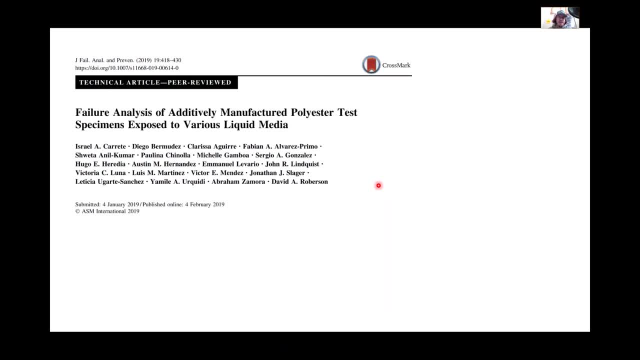 One was polylactic acid, The other one is PETG, So these are off the shelf- additive manufacturing filaments, basically- And we exposed them to different liquid media And this was all off the shelf. So we exposed it to stuff like vinegar and Coke and stuff like that And it's a pretty good article. 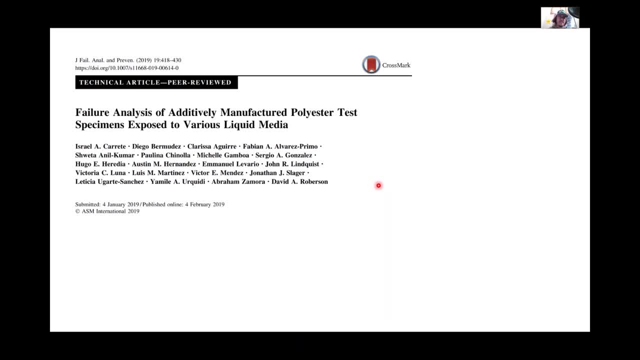 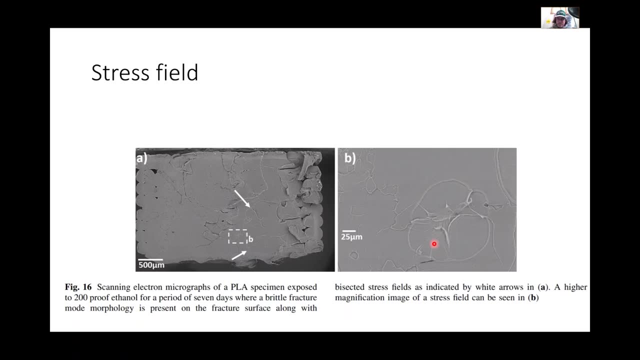 I will probably post this on Blackboard as well if you want to have a look, But I'll take. excuse me there my phone was ringing. The next images come from this article, So stress-filled. So here's kind of another example of a stress-filled And you can kind of almost see. So we had really good printing. 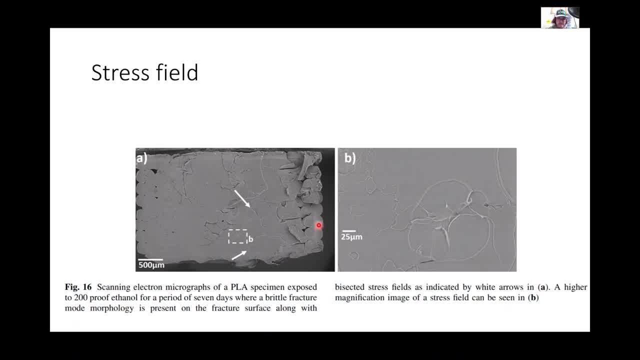 parameters when we printed this stuff. There's not many voids. I've talked sometimes about the heat dissipating off the air. You can see the edges of a 3D printed structure So you don't get the polymer diffusion And so in the edges. 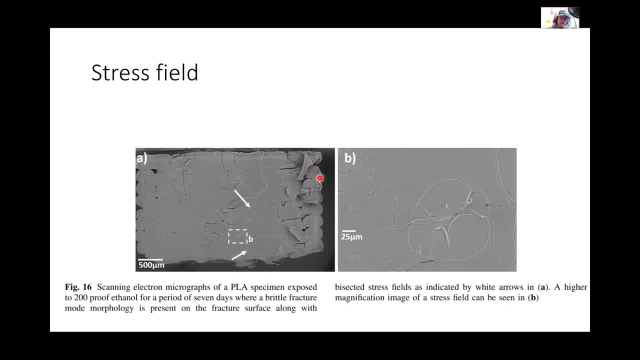 we kind of see some voiding And we don't really see that in the interior, depending on what this raster pattern was. This is actually the perimeter. So we printed with a perimeter And if you're familiar with 3D printing, you know exactly what I'm talking about. If you're not familiar with 3D printing, I'll put it in. 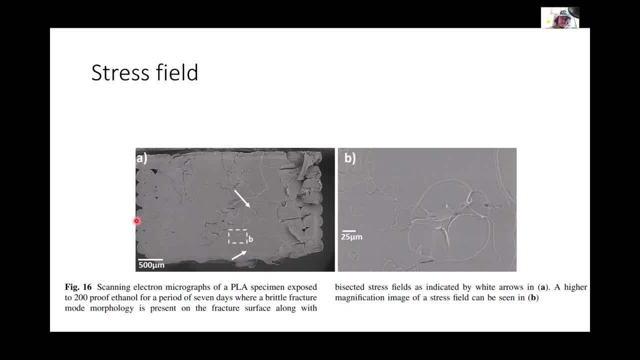 really, really layman's terms. This pattern is not representative of the entire specimen, I think. So there is a perimeter first, and then, even if it was the same, it doesn't matter. there's the perimeter first, And then it goes and fills in the interior. So does the perimeter first. So if you print with a 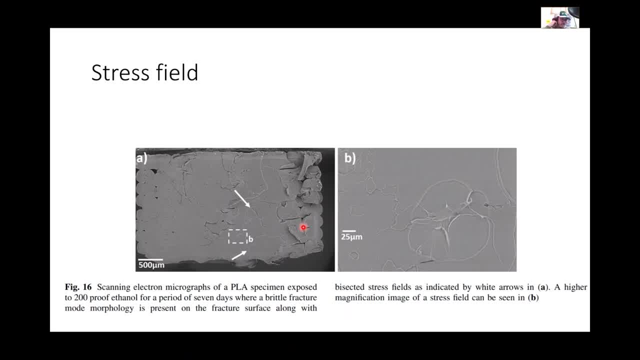 perimeter. you can kind of run into some problems like this- but that's not the full thing here, What we have- and you can kind of see traces of the layer here and it extends in. So we see the trace of the layer here and then we see there's some defect caused by the inner layer. So it's an inner layer but there's a 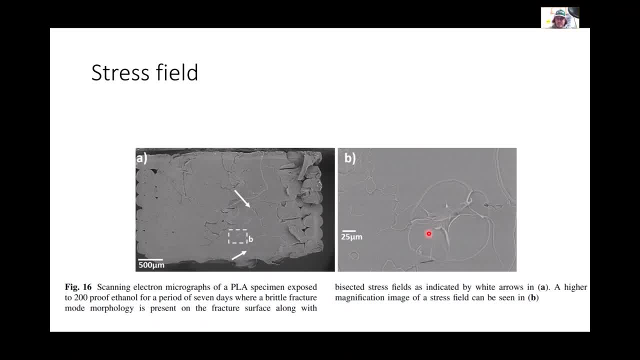 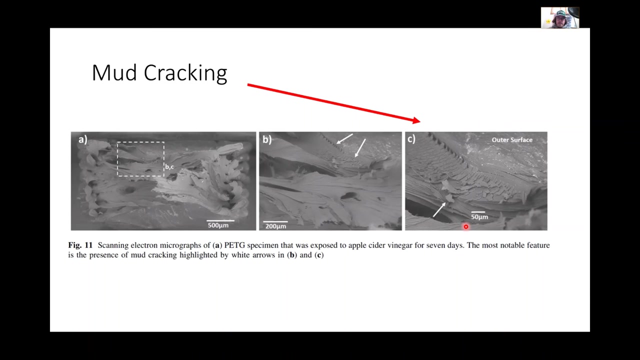 layer defect led to the manifestation of a stress field, and again pretty close to circular structure. actually we see kind of two intersecting stress fields together, both caused by interlayer defects, basically due to the printing process. mud cracking is one that's really kind of cool. mud cracking's actually caused by molecular damage. 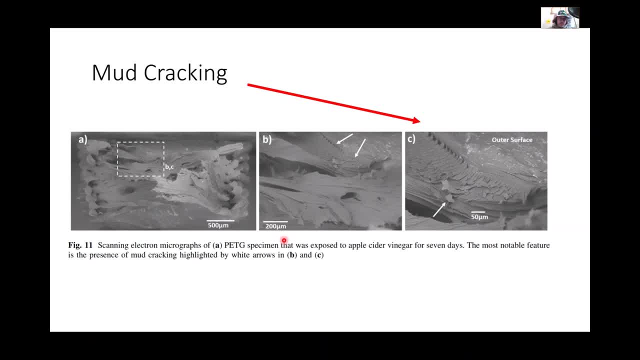 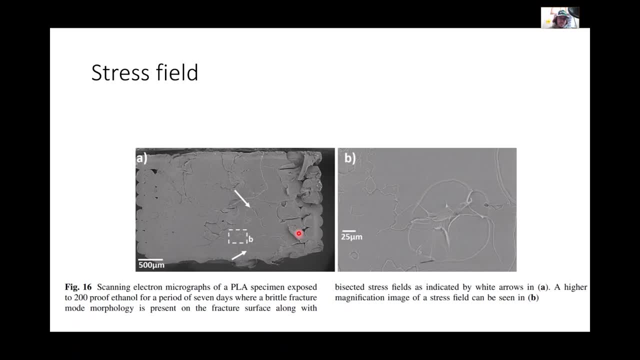 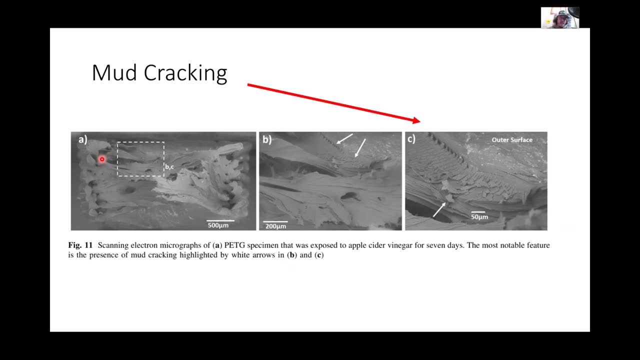 and so one thing i'll point out: this is a pet g, so this one was pla, so you notice that it's still pretty flat. there's not that much deformation due to the tensile test. pet g it's polyethylene tetraphalate, so polyester, but it's a plasticized with uh, with um, um, what's it plasticized with what? 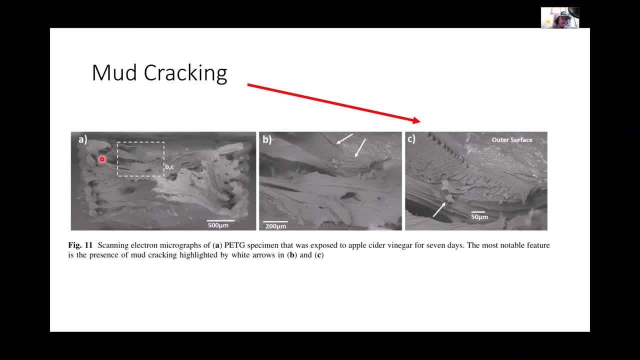 is the g glycol and ethylene glycol. excuse me, had to remember and you saw me, uh, struggle to remember, but ethylene glycol is a plasticizer, so it is a much more ductile material. so you see, there's some necking occurring before final rupture. quite a bit of necking, actually. this would have been a more. 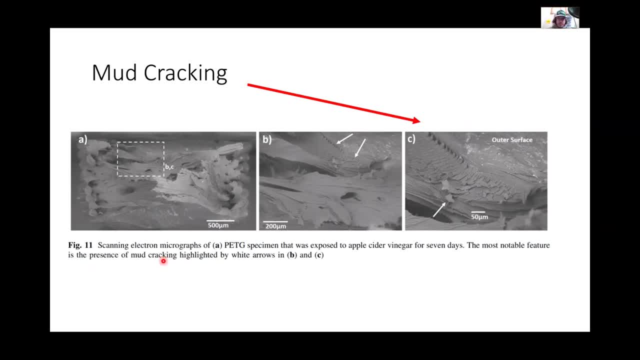 rectangular looking structure and we see this interesting feature here. this is called mud cracking and this mud cracking is due to basically molecular breakdown, molecular damage. it's irreversible. and so some molecular damage is irreversible and some molecular damage is irreversible to polymers is reversible. so if you've overexposed it to moisture you can kind of bake it off and 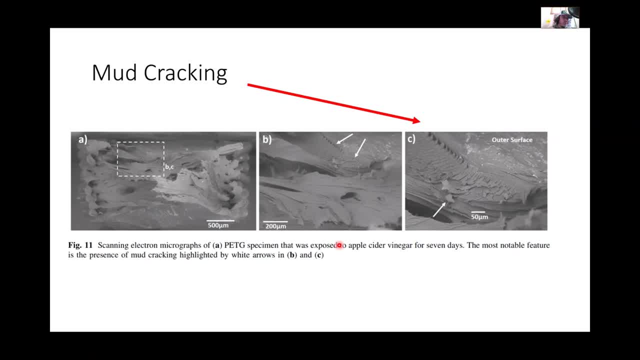 and kind of heal your material, if you will. so you can, you can warm it up, and different polymers, depending on what they are, will even have drying schedules and and so you can kind of heal the material, remove the moisture and especially if you're going to reprocess it, 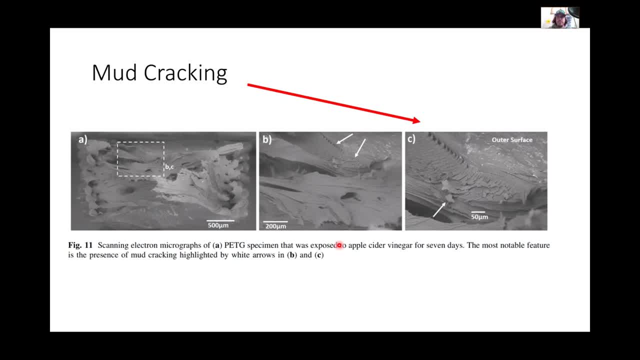 right if you're going to uh, melt it again or injection molded or whatever, but when you have stuff like this, like mud cracking, you've severely damaged the material, and this was due to apples. this was exposed to apple cider, apple cider vinegar. so it's actually kind of interesting, because sometimes apple cider 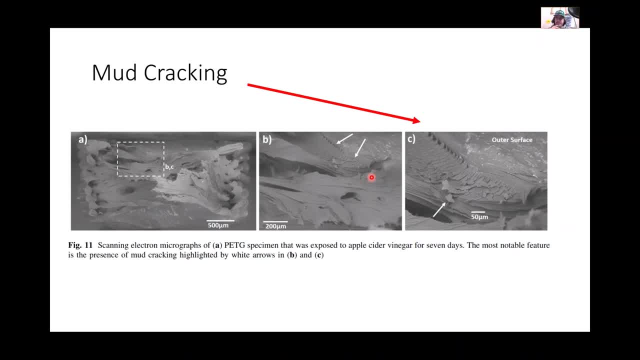 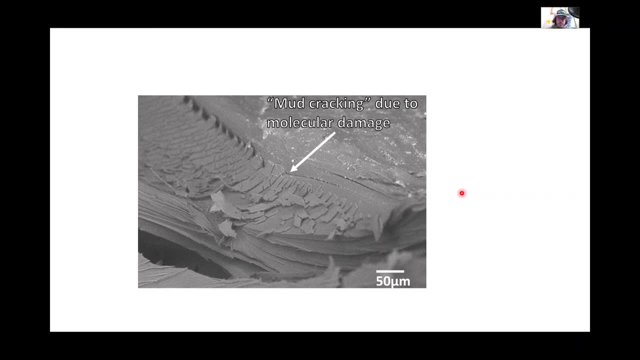 vinegar is sold in in pet bottles, not pet g, so the plasticizing seemingly made it more susceptible to degradation due to exposure to apple cider vinegar. but anyway, mud cracking and i really like these features. i have a bigger one of the of the same um, a bigger image of the same feature. 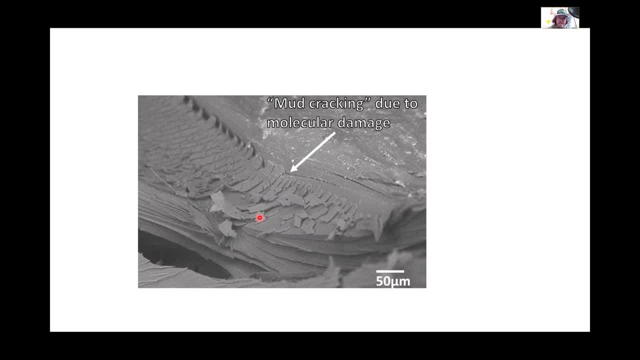 and you kind of see it's just flaking off and you can really appreciate the damage that was done to the material by exposing it to the liquid media it was exposed to, in this case apple cider vinegar, other things to kind of look at. again, this is pet g. this was exposed to. 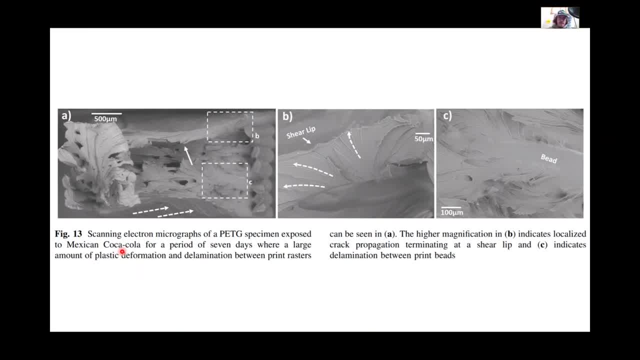 mexican coke and um very specific. there a lot of plastic deformation occurred and um. there's a other story, but i'll focus mostly on the um, on the, the key um fracture surface. i want to show which is a sheer lip. it's kind of this deformation at the end of uh, at the end of the failure, or the final. 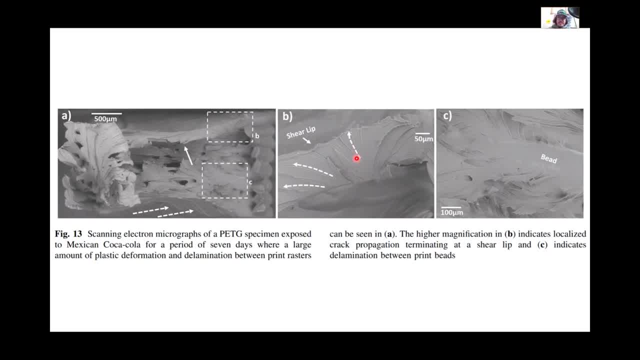 rupture for at least this crack interface um the sheer lip, and so that's another feature to look at. i didn't title the slide because i had it labeled on the on the picture. um, this is another thing i kind of want to show. so this is pet g again, you can tell a. 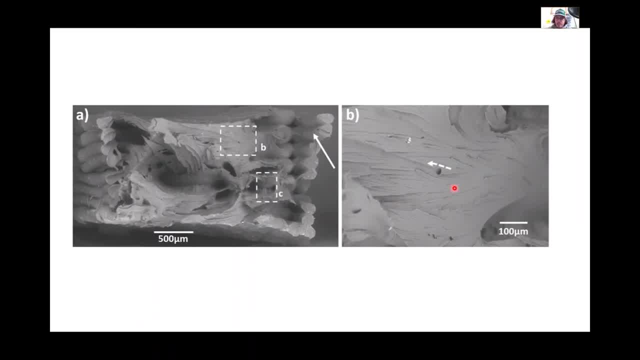 lot of plastic deformation, but this void here did not play a part in the failure of this material. basically is what i'm trying to show, and so not all defects in a polymer specimen play a role in the overall failure. and, um, i've kind of argued this with people now and again, but this is due to 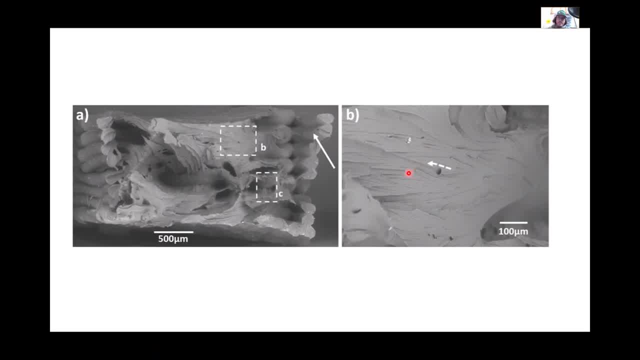 viscoelastic flow. if it's big enough, okay it'll. it'll cause some problems and we've seen that earlier in this lecture. so it's almost um um like a critical defect size for a material. but viscoelastic flow kind of remedies the presence of defects in some cases- not always, but in some cases. 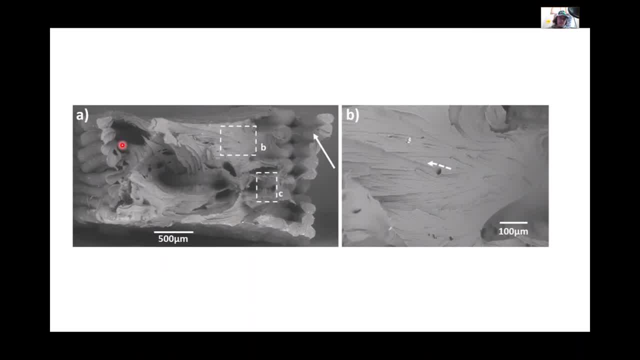 and this underwent a lot of plastic deformation before it failed. but this void didn't really have much to do with the overall failure, so the crack kind of propagated around it and i have other examples and other papers that i can share with you if you're interested. 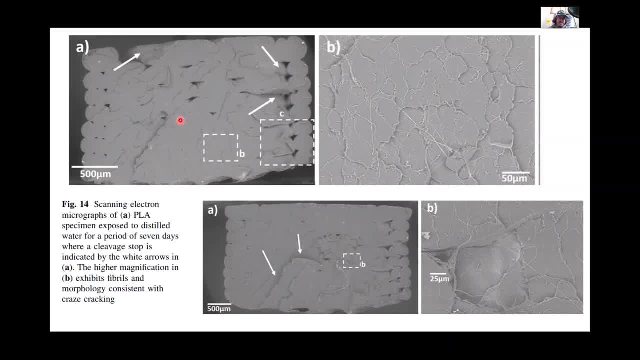 this is pla, so again a ductile, not a ductile failure, more of a brittle failure. this is a really good example of fibrils on the fracture surface and so the fibril layer areas are localized. but, um, again, fibrils can occur, or fibrils do occur.